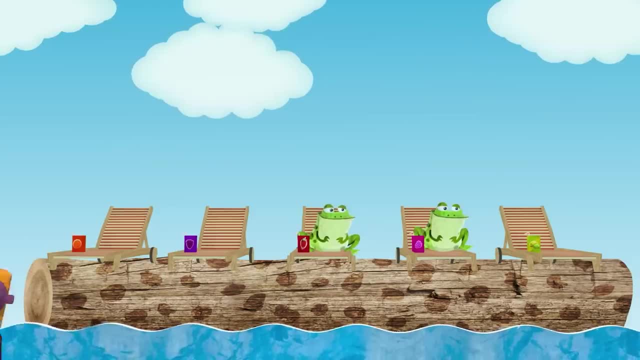 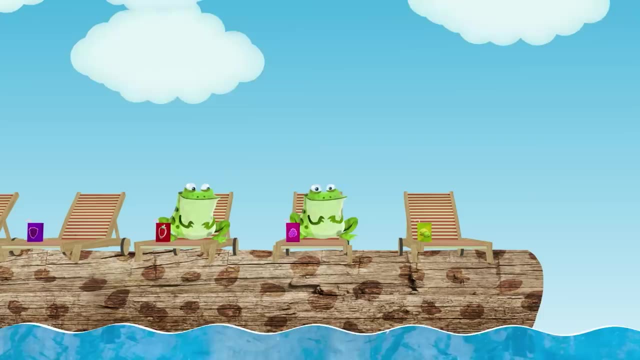 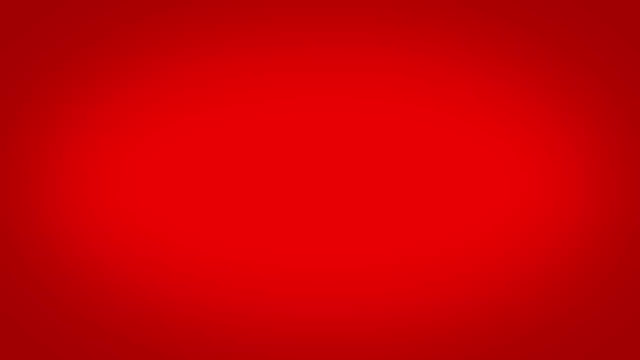 1, 2. Two little speckled frogs sat on a speckled log Eating some most delicious bugs, yum, yum. One flew off into space- you should have seen her face. Now there is one green speckled frog, blub, blub. 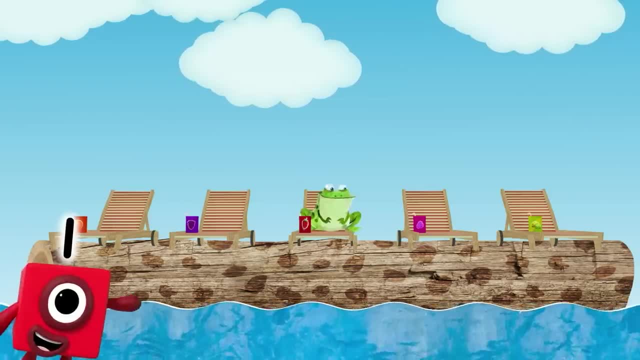 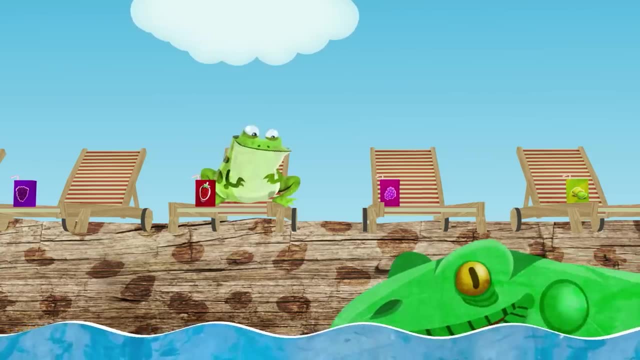 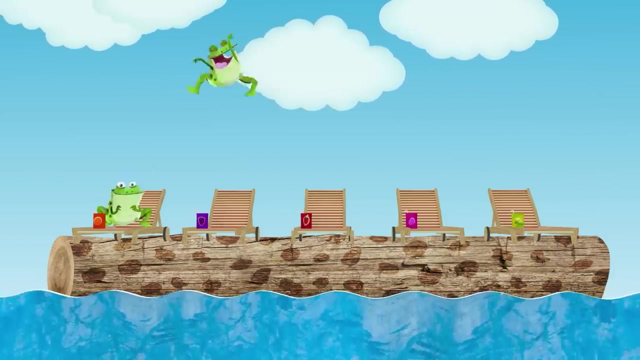 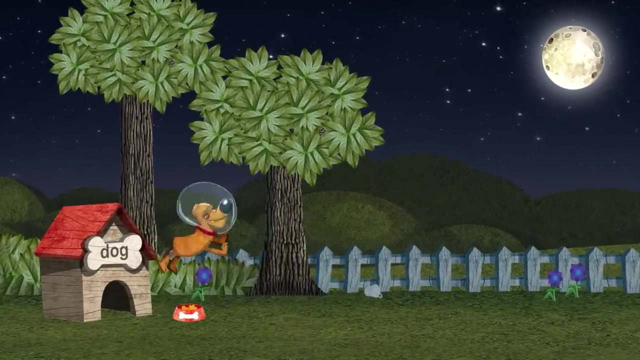 1. One little speckled frog sat on a speckled log Eating some most delicious bugs- yum, yum. He saw a crocodile and jumped about a mile. Now there are no green speckled frogs. Zoom, Zoom, Zoom, we're going to the moon. 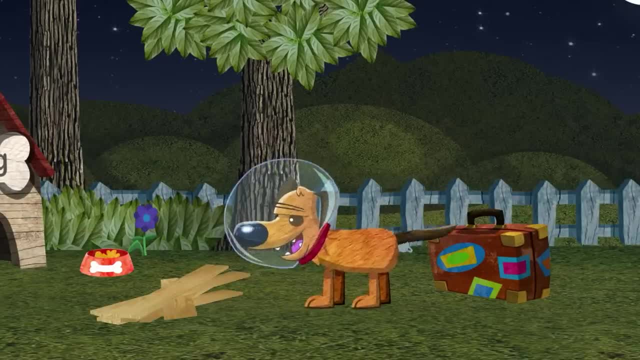 Zoom, zoom, zoom, we're going very soon. If you want to take the trip, climb aboard my rocket ship. Zoom zoom zoom, we're going to the moon. Zoom zoom, zoom, we're going very soon. Zoom zoom, zoom, we're going very soon. 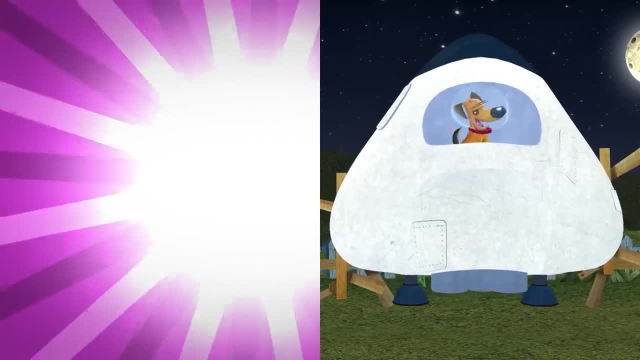 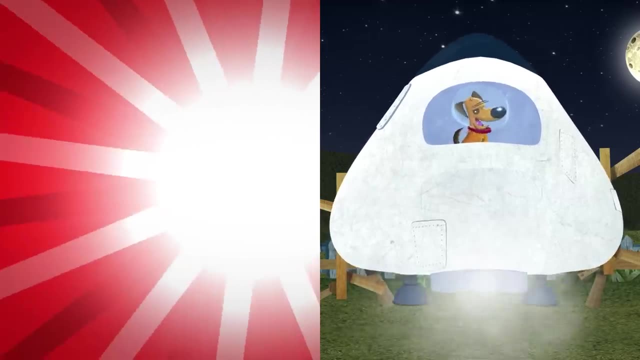 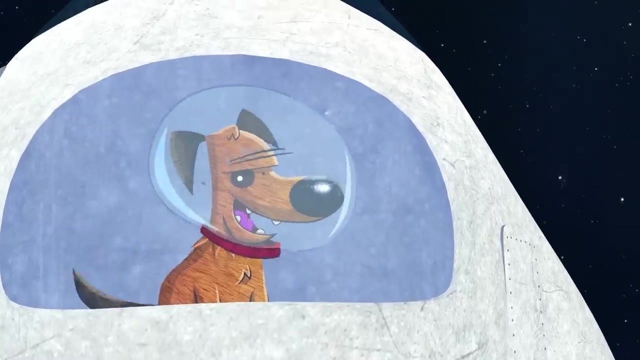 10,, 9,, 8,, 7,, 6,, 5,, 4,, 3,, 2, 1. Zoom, zoom, zoom. we're going to the moon. Zoom, zoom, zoom. we're going very soon. 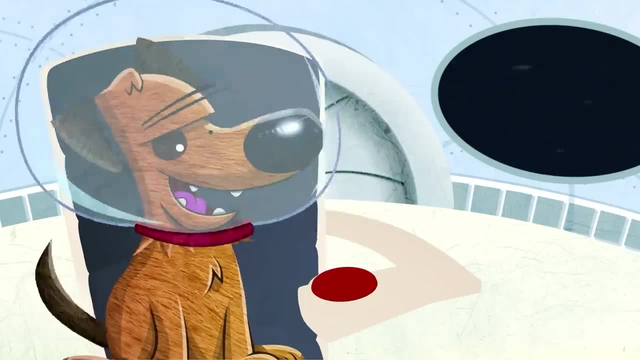 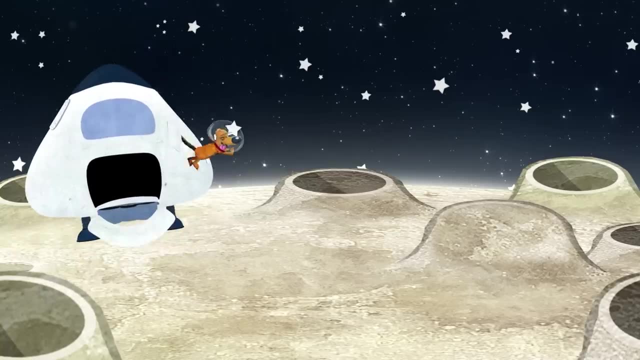 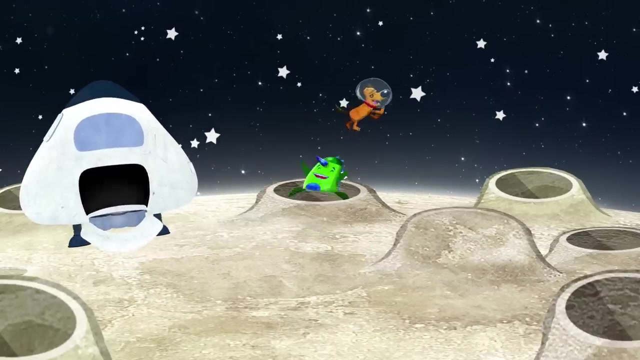 If you want to take the trip, climb aboard my rocket ship. Zoom, zoom, zoom. we're going to the moon. We're gonna have a celebration now we're here, Even though there's not a lot of atmosphere. I wonder if these aliens know anything about us. 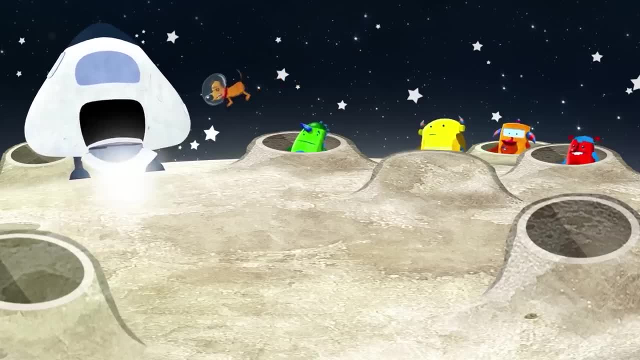 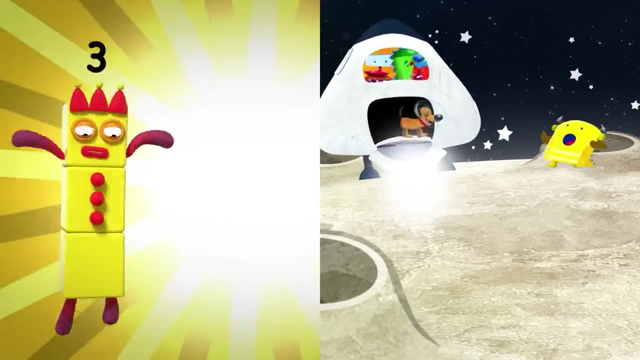 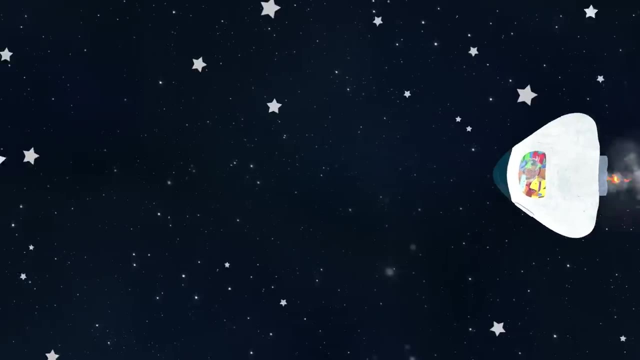 Wait, I think the rocket's taking off without us. 10,, 9,, 8,, 7,, 6,, 5,, 4, 3, 2, 1, Zoom, zoom, zoom. we're heading back to base. 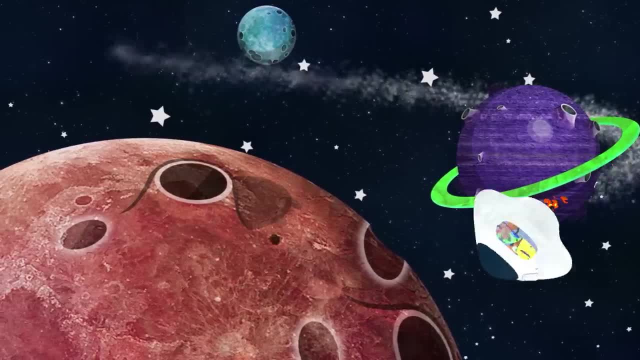 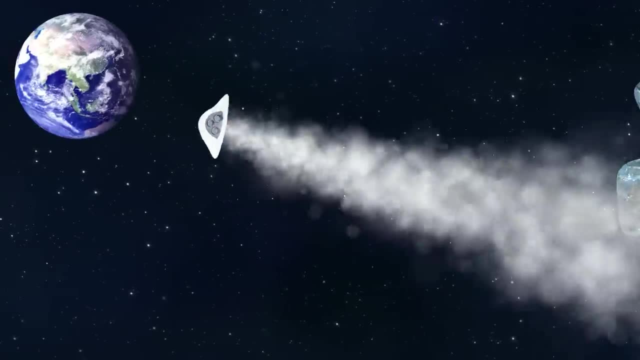 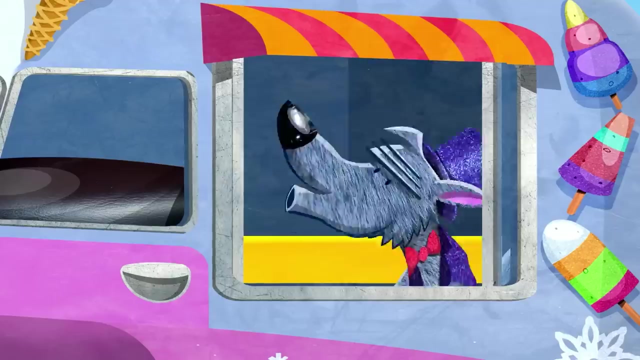 Zoom, zoom, zoom. we're going to win the race. If you want to hitch a ride, catch us up and step inside. Zoom, zoom, zoom. we're heading back to base, Cause we're running out of space. Scoop a scoop, a scoop of vanilla. 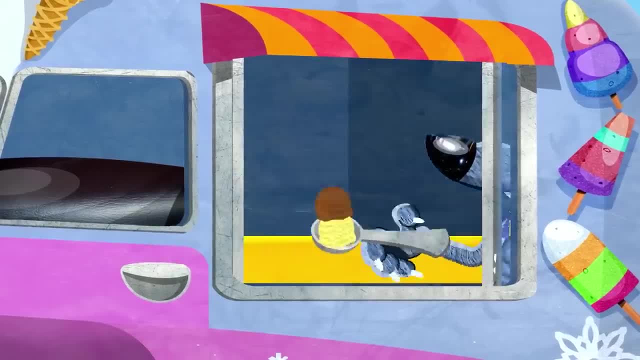 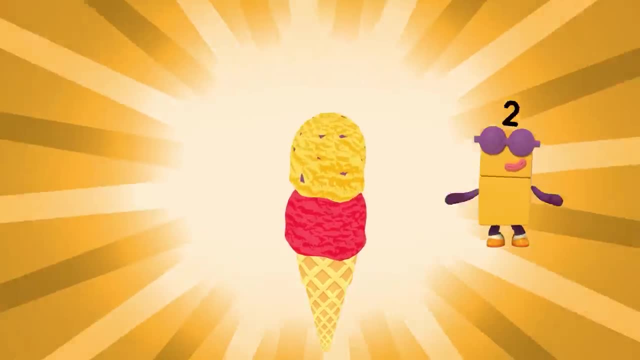 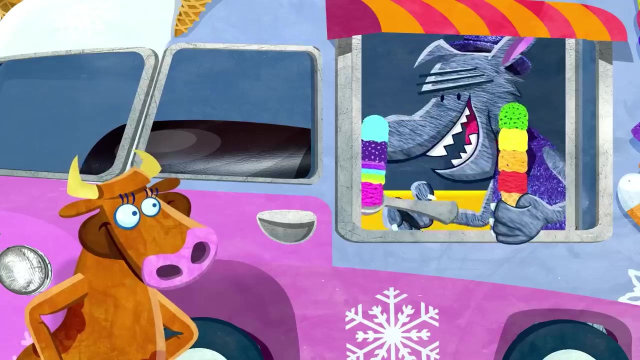 Scoop, a scoop, a scoop of chocolate Scoop, a scoop, a scoop of strawberry And a scoop of mint chocolate chip. One scoop, two scoops, Three scoops, four scoops. Everybody wants more scoops In a great big waffle cone. Five scoops, six scoops. 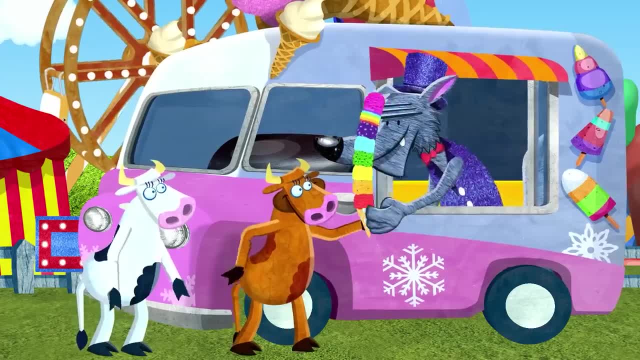 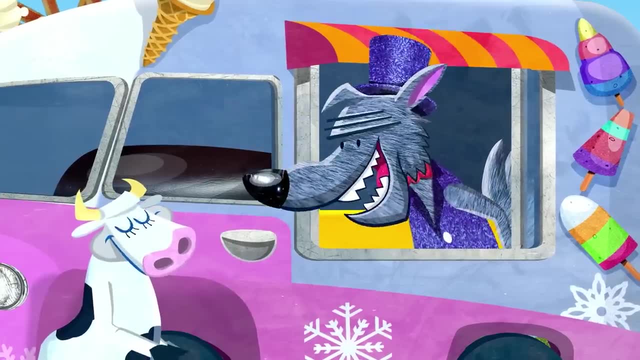 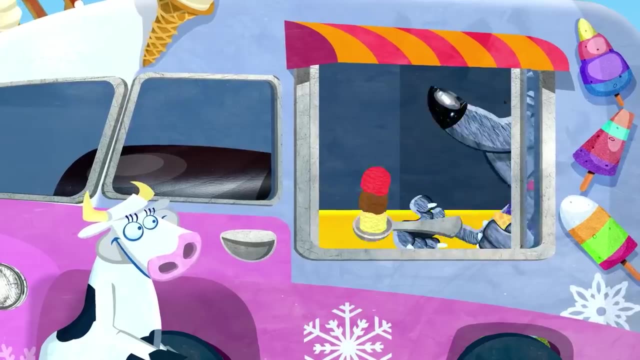 Seven scoops, eight scoops. No one ever ate eight scoops. It's the biggest ice cream The world has ever known. Scoop a scoop, a scoop of vanilla. Scoop a scoop, a scoop of chocolate. Scoop a scoop a scoop of strawberry. 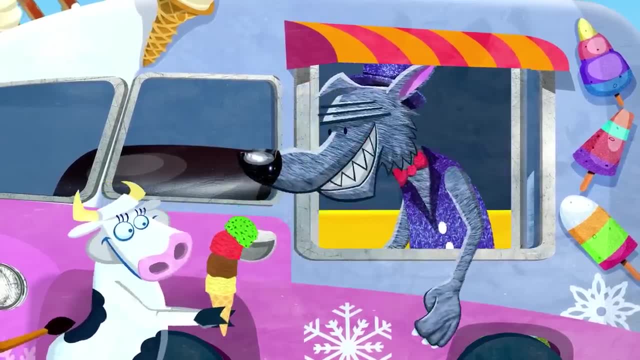 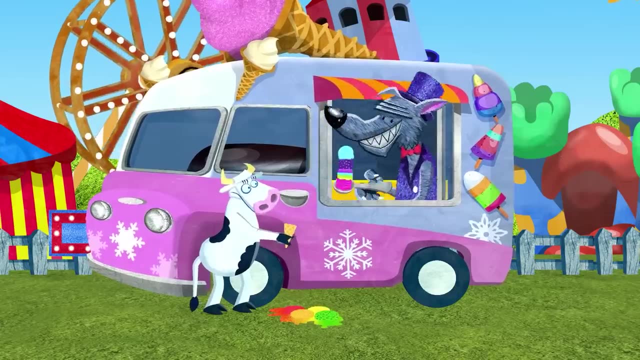 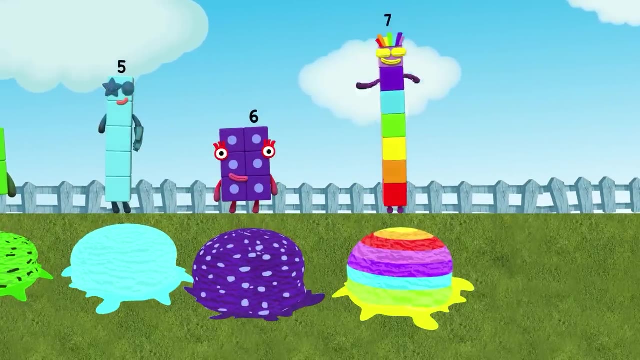 And a scoop of mint chocolate chip. One scoop, two scoops, Three scoops, four scoops. I think we're gonna need more scoops. They're all melting, that's no fun. Five scoops, six scoops, Seven scoops, eight scoops. 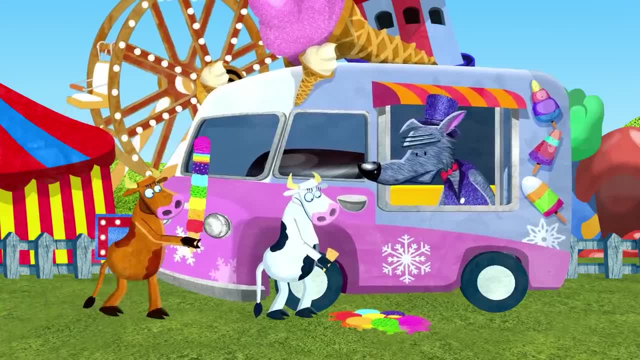 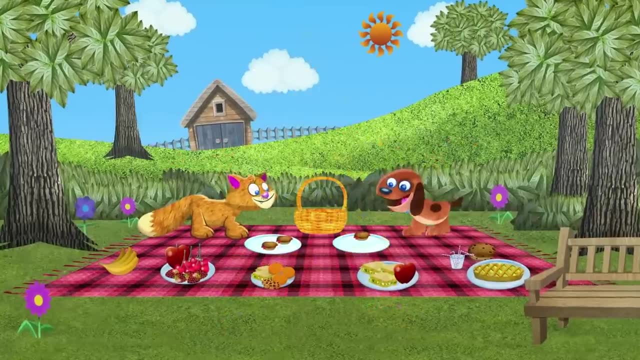 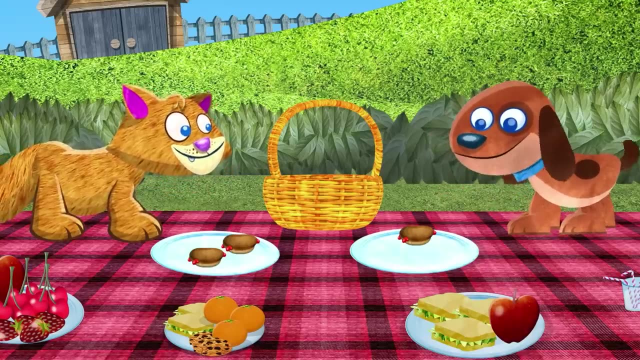 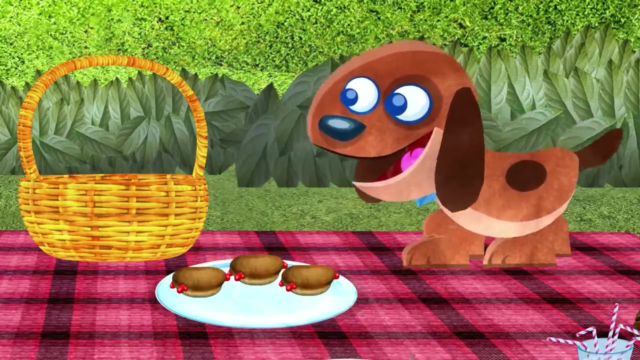 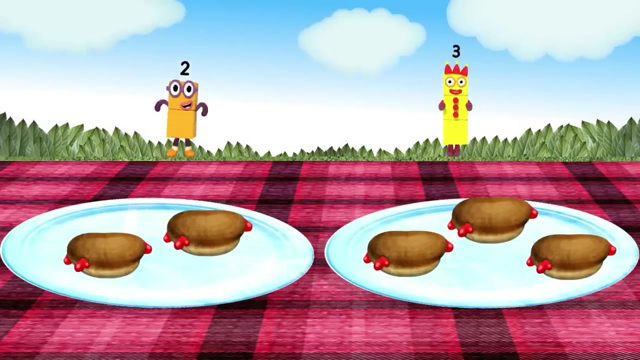 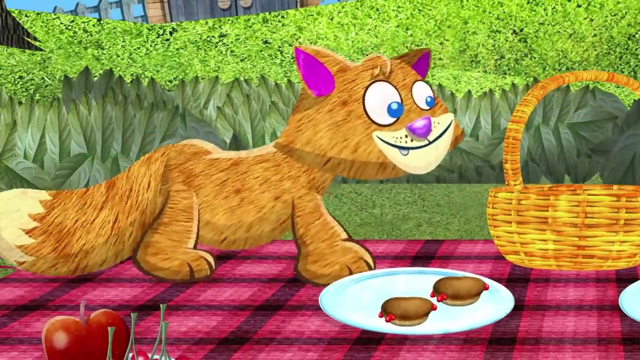 I bet you wanted those eight scoops. Maybe next time you're gonna need more scoops. Maybe next time you won't leave them in the sun. So I've got more scoops than you. If you add two scoops, Then you've got four scoops. 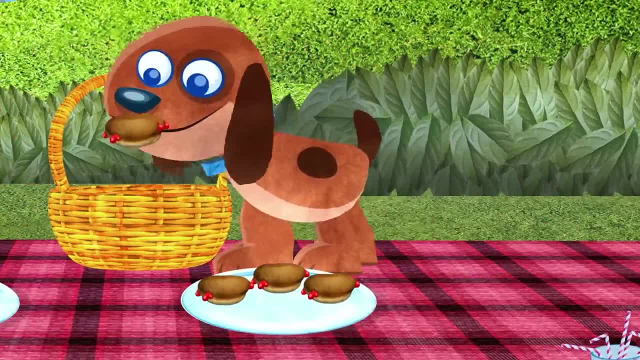 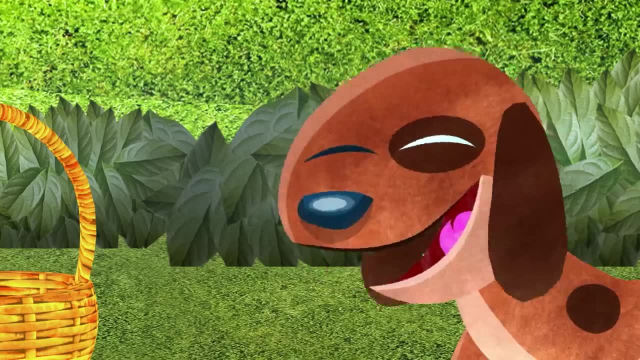 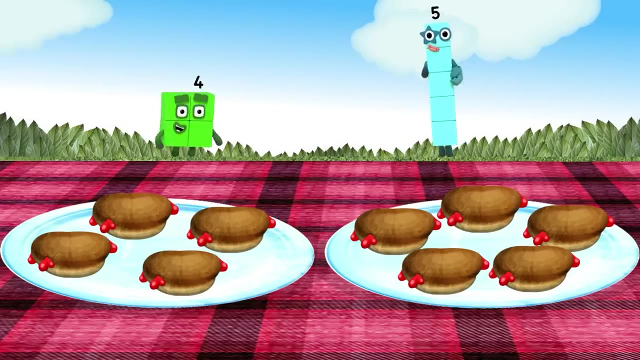 And four is more than my three, So I add two scoops. Now you've too few scoops, Cause I've got five scoops. That's more scoops than four scoops, Cause four is one more than three And five is one more than four, So I've got more scoops. 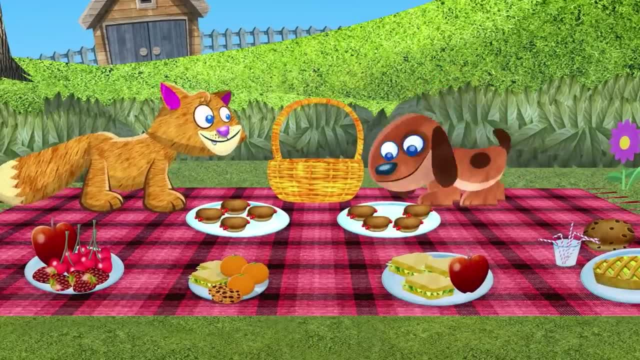 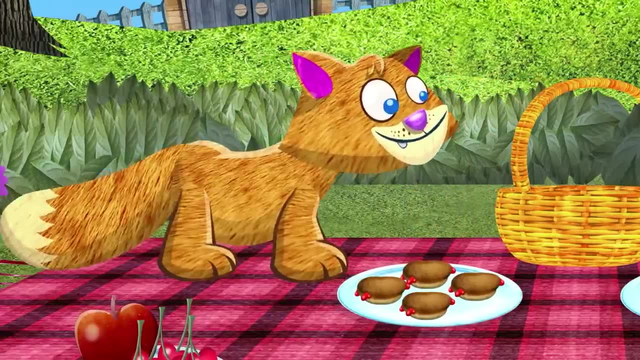 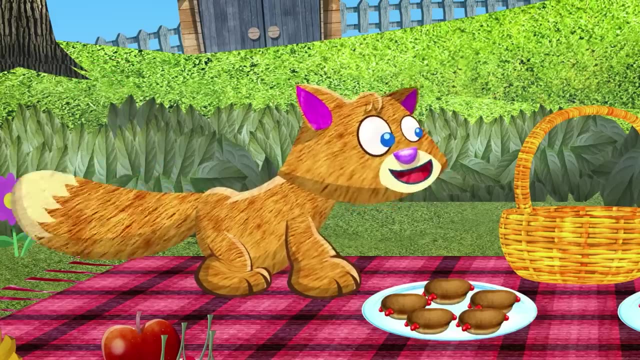 Once more. If I eat one, I'll have four, like you. Then we'll both be the same. But I've had one bun And you've had none. Oh, this is a difficult game, So I'll give you one bun. Now you've got five buns And I'll be happy with three. 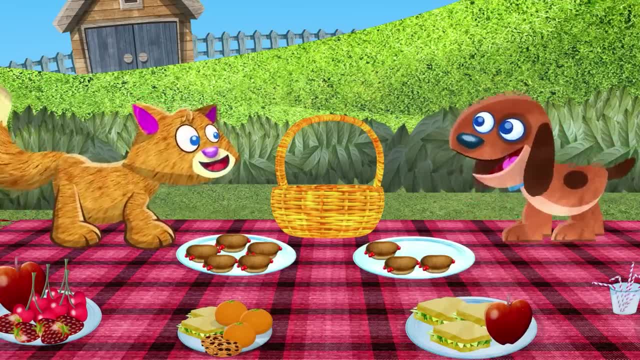 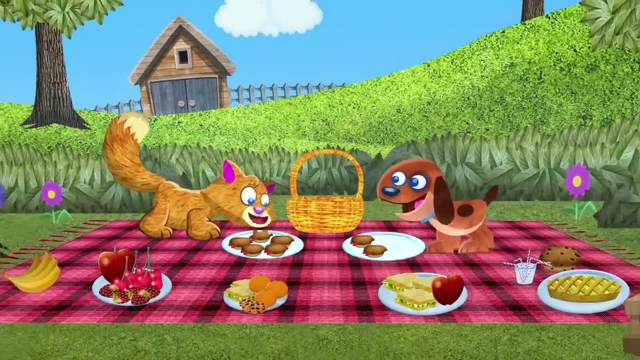 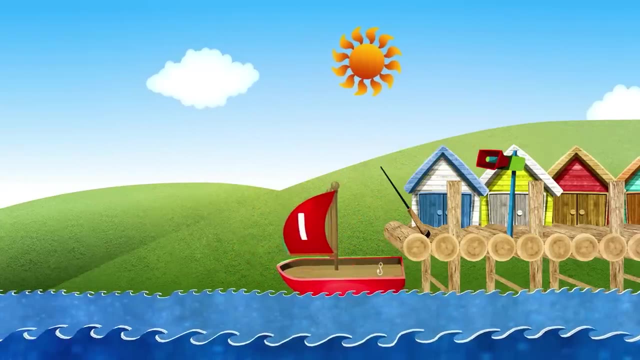 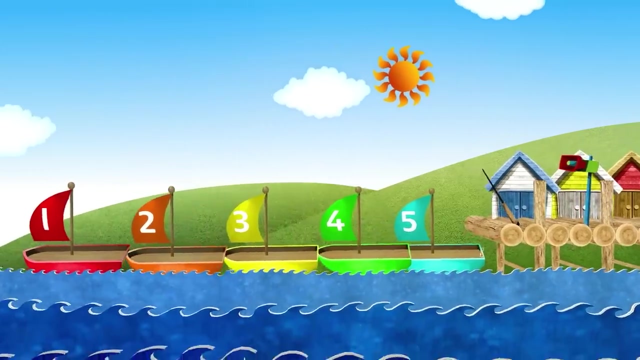 Cause sharing's the done thing. This is the fun thing, The one thing we can agree. We both like eating Buns for tea. Five boats sail away. One, two, three, four, five, Five little boats out in the bay: One, two, three, four, five. 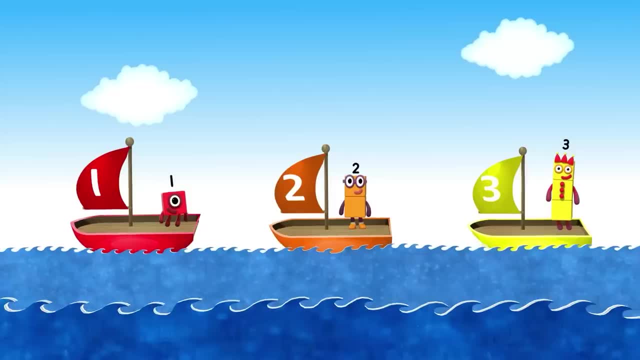 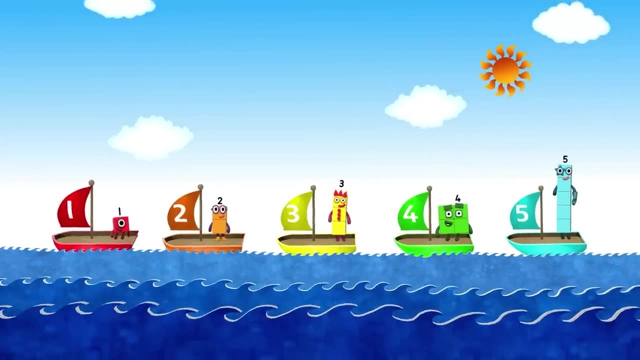 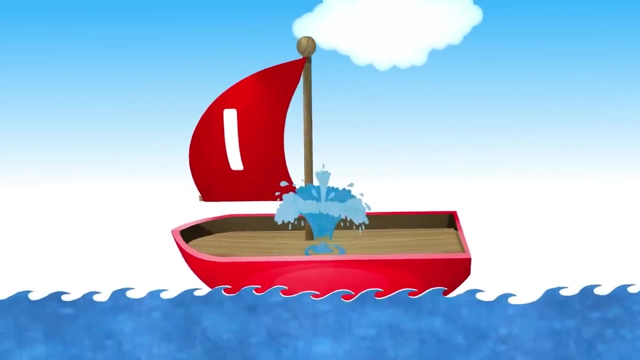 First comes one, then two, then three, Three boats sailing out to sea. Four and five are next in line. Don't those five little boats Look fine? Suddenly, one springs a leak. Now it's on a losing streak. Two goes fast, Three pulls past Two, three, one, four, five. 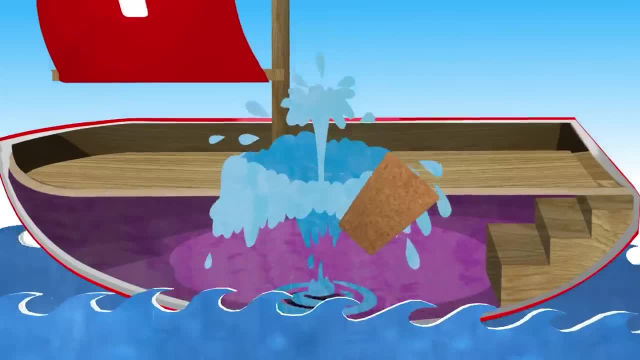 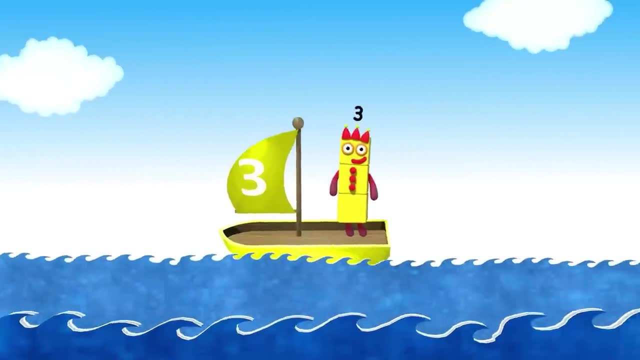 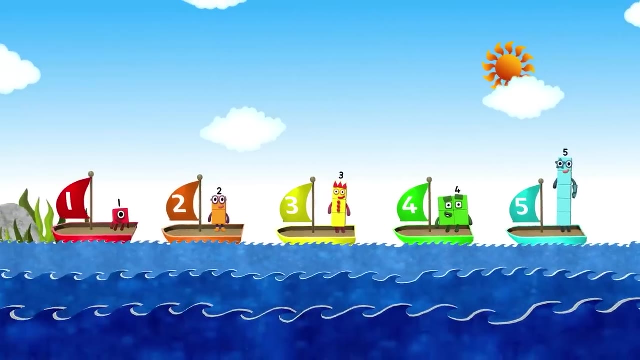 Hang on, That's wrong Wait Time to set this straight. First comes one, then two, then three, Three boats sailing out to sea. Four and five are next in line. Don't those five little boats? Don't those five little boats Look fine? Suddenly, one boat gets stuck. 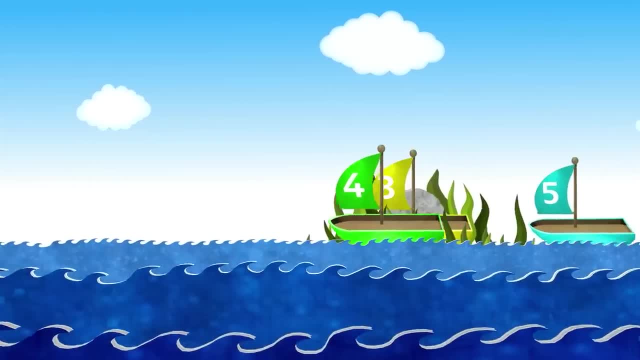 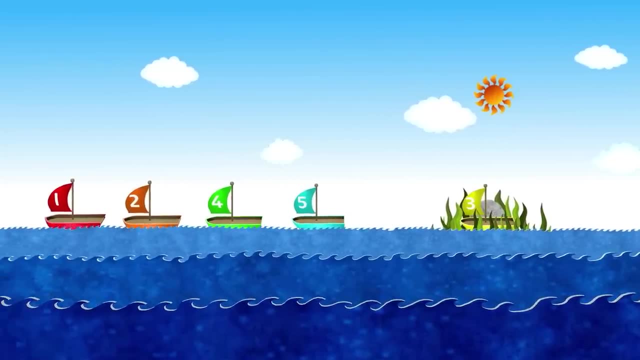 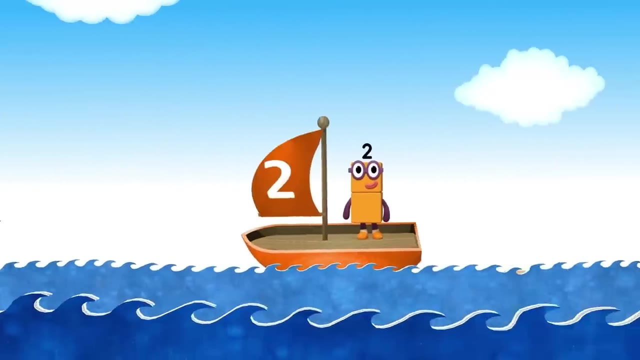 What a piece of rotten luck. Four goes fast, Five pulls past One, two, four, five, three. Hang on, That's wrong. Wait Time to set this straight. First comes one, then two, then three. Three boats sailing out to sea. Four and five are next in line. 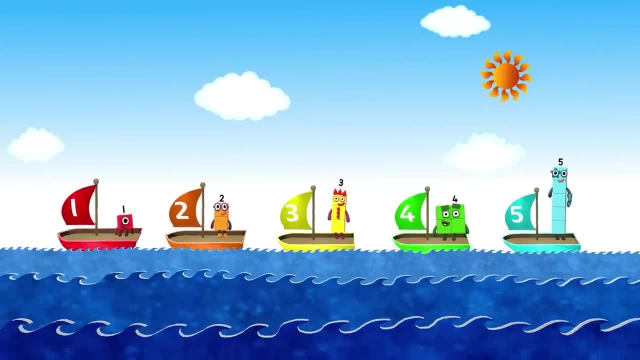 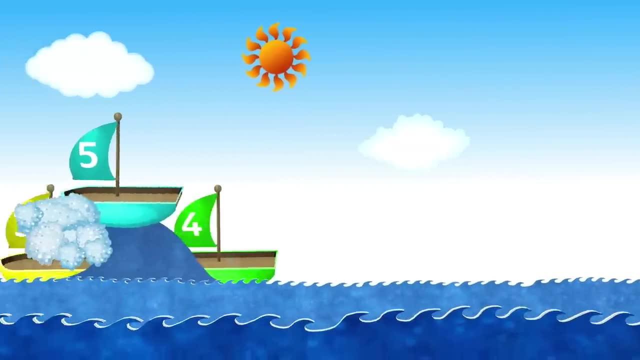 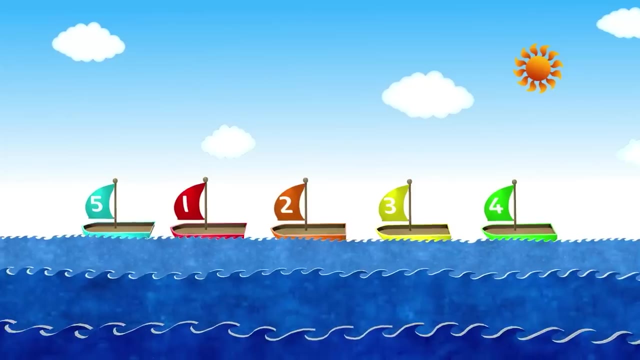 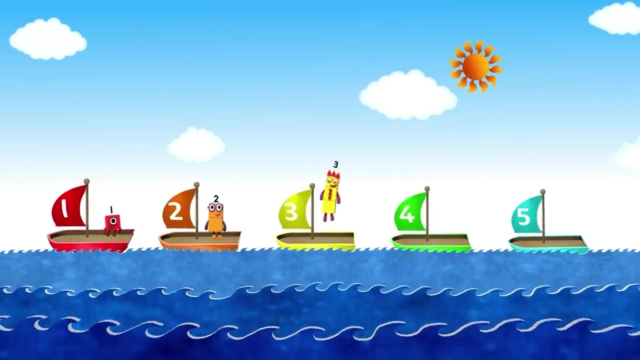 Don't those five little boats Look fine. Suddenly one meets a whale, Gets flipped by a massive tail, Goes so fast, Flies right past Five. one, two, three, four. Hang on, That's wrong. Wait Time to set this straight. First comes one, then two, then three. 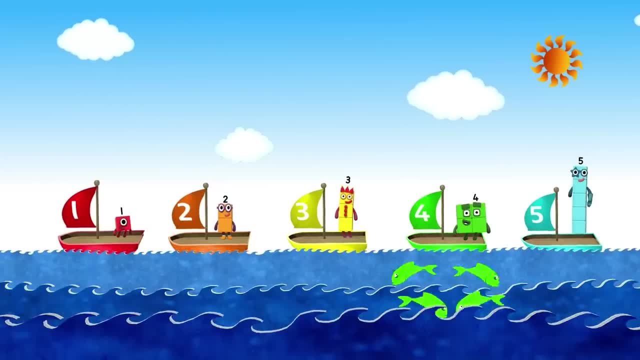 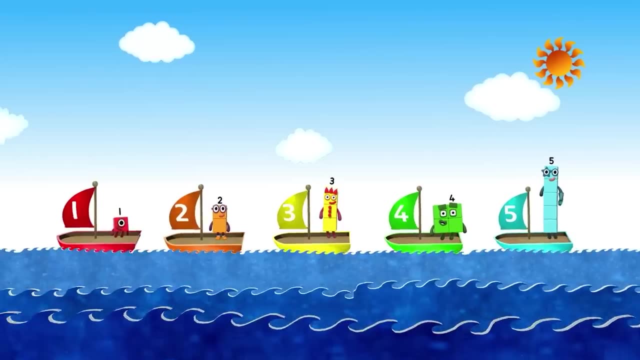 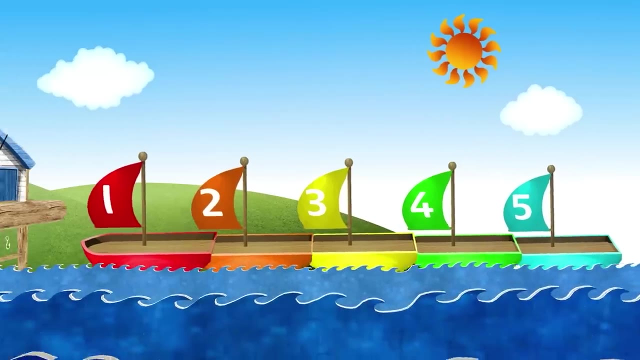 Three boats sailing out to sea. Four and five are next in line. Don't those five little boats Look fine. Five boats sail away. One, two, three, four, five. Five little boats out in the bay. One, two, three, four, five. 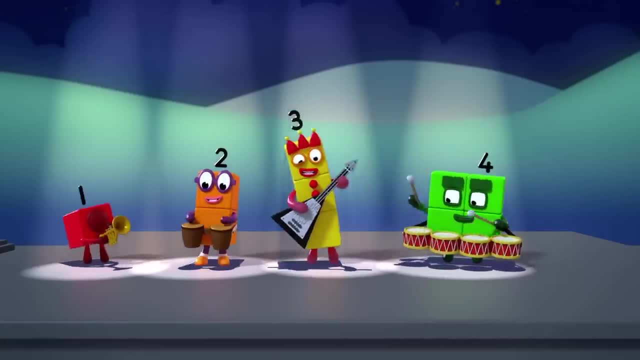 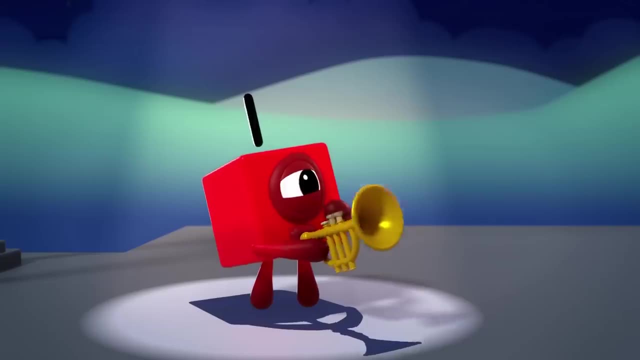 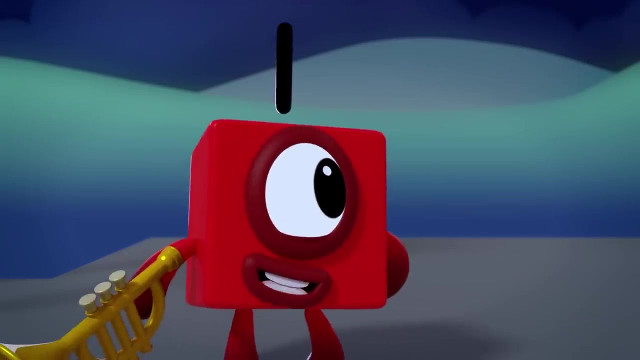 Hang on. One, two, three, four, five. Three boats sailing in one, two, three, four. Three boats sailing in one, two, three, four. Ah, Two, slow, You're too fast, I can't keep up. Stop. That was one awful sound. 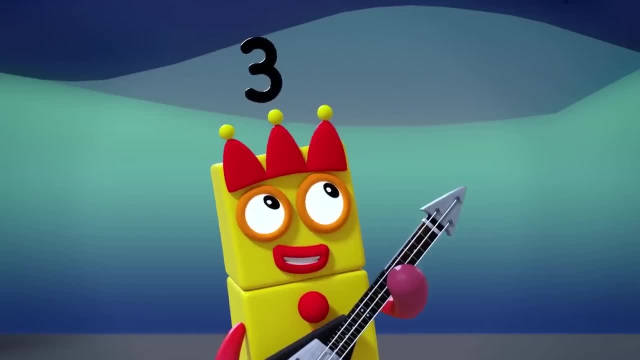 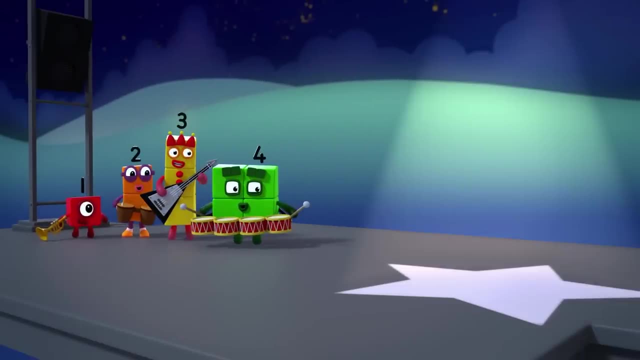 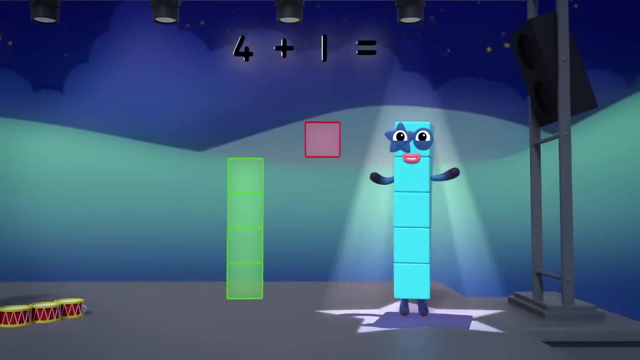 We need someone to sort us out. Ah, A shooting star Make-A-Wish. Oh, it's star-shaped. Who's it for Me? Well, I'm the biggest, I'll go first. Four Plus one equals five. I am five. 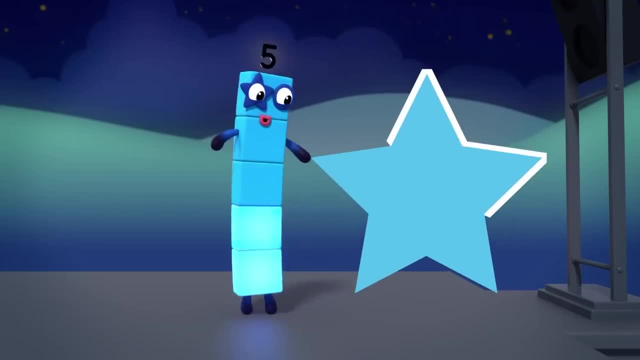 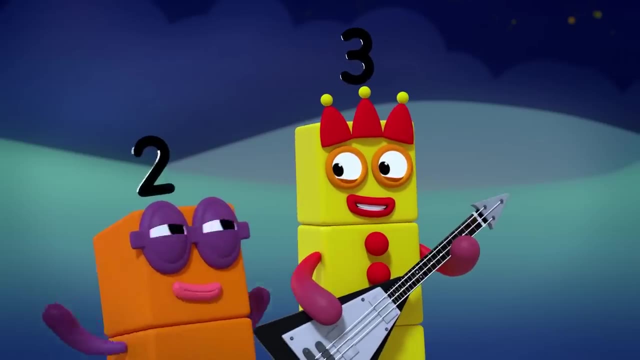 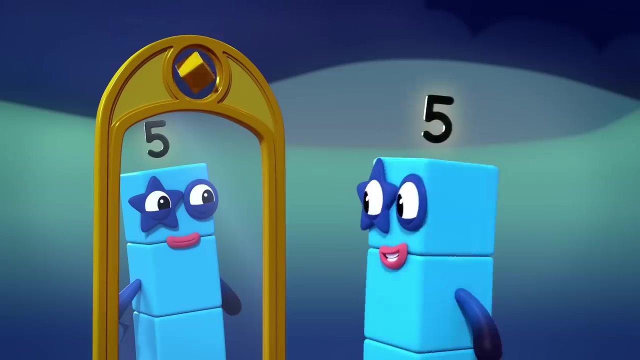 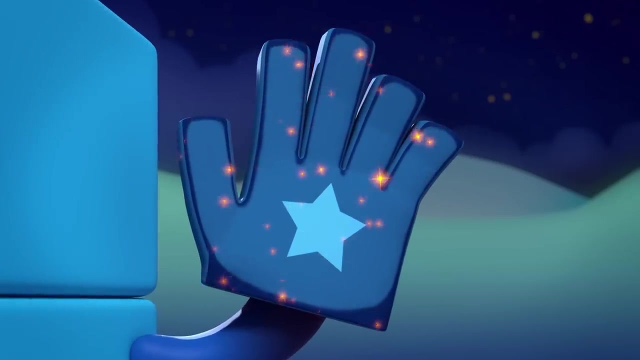 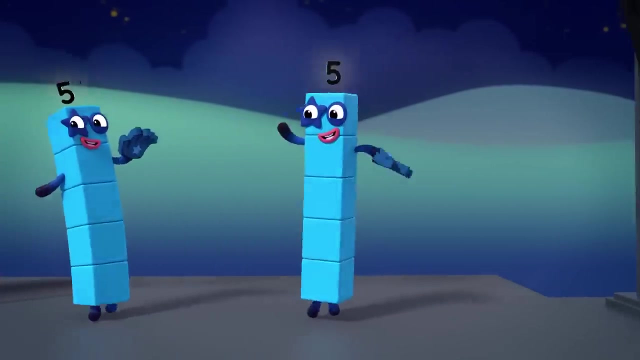 I feel so alive. One, two, three, four, five, Five points, Oh, a star is born. I don't know about that. Take a look, High five, High five. Oh, A big hand for you, High five. 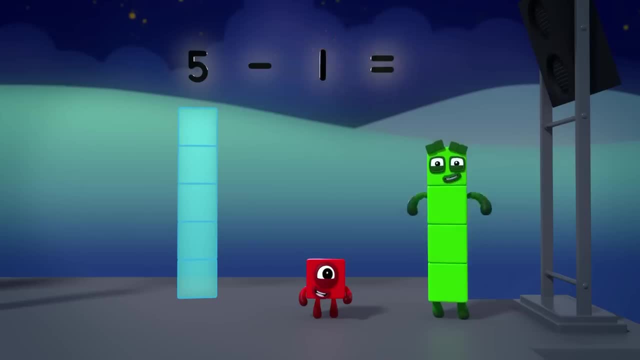 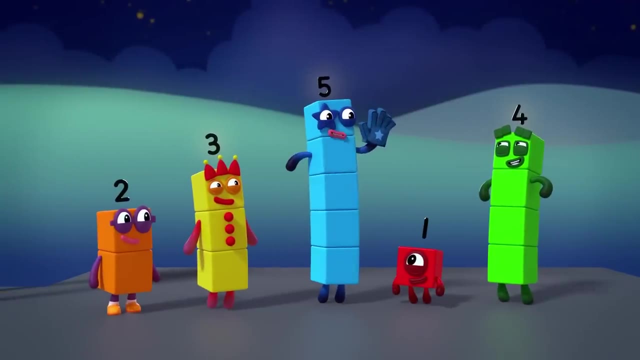 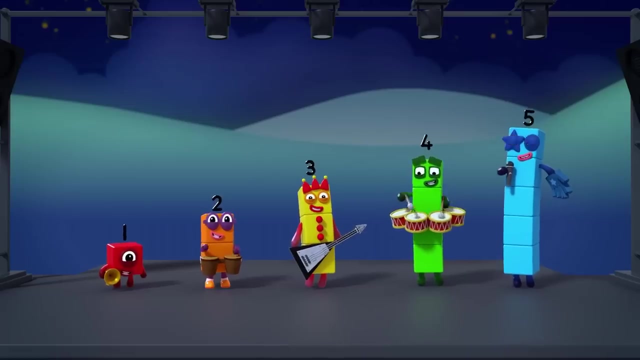 Five minus one equals four. Ooh, And who are you? I'm five And you can count on me To get this party started. Five members in my band: One, two, three, four, five, Five fingers in my hand. 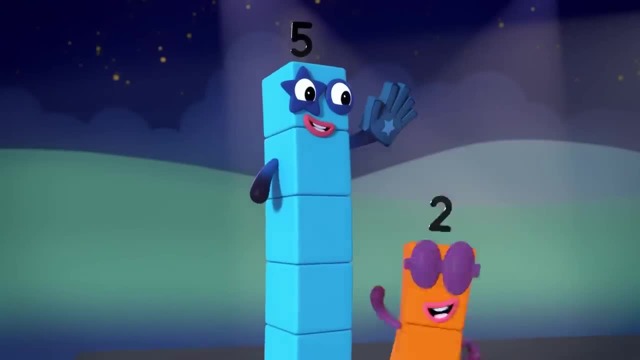 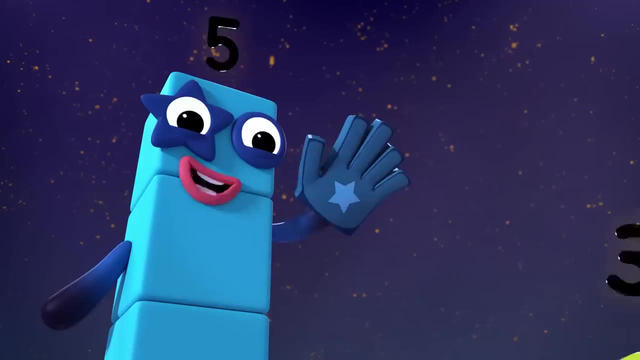 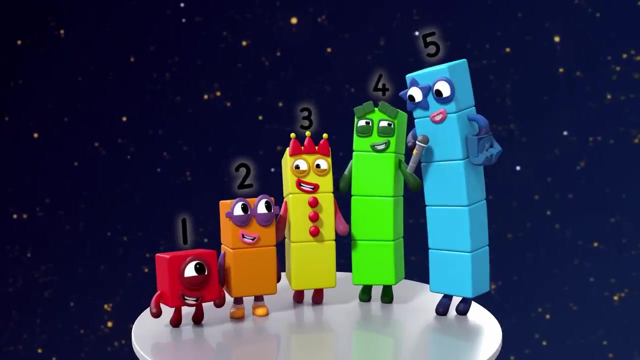 One, two, three, four, five. High five, High five, High five. I'm gonna let you pass Hi-five Down low too slow. High five. Ooh, I feel so alive. You know that you've arrived When you're with number five. 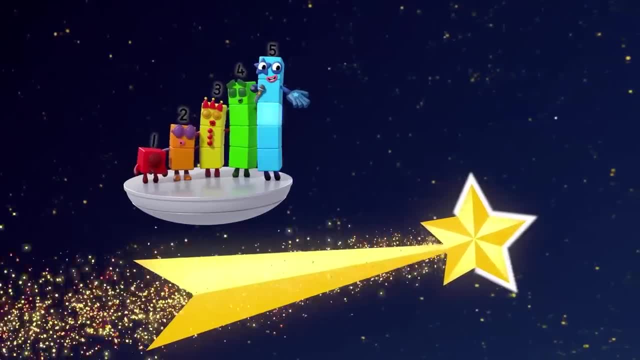 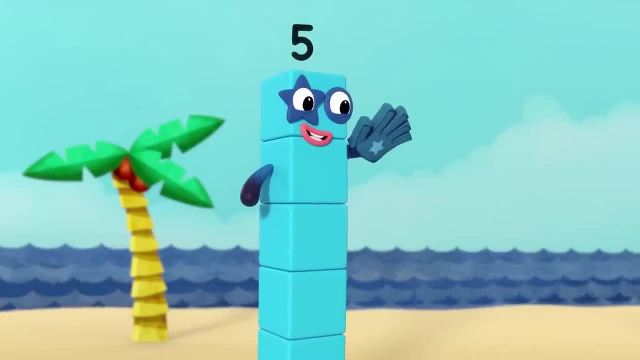 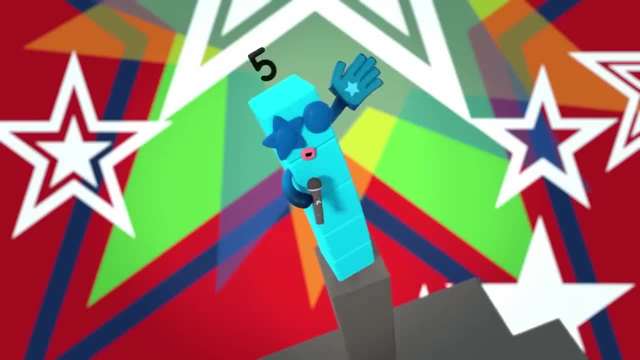 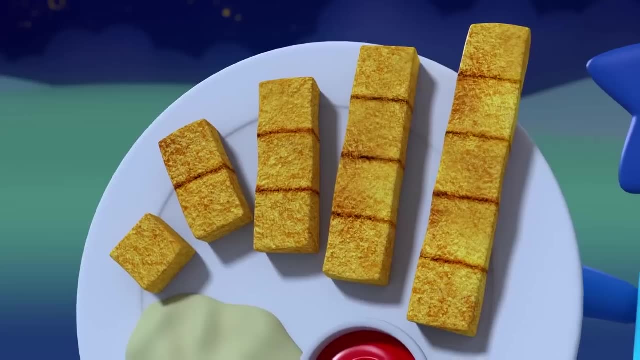 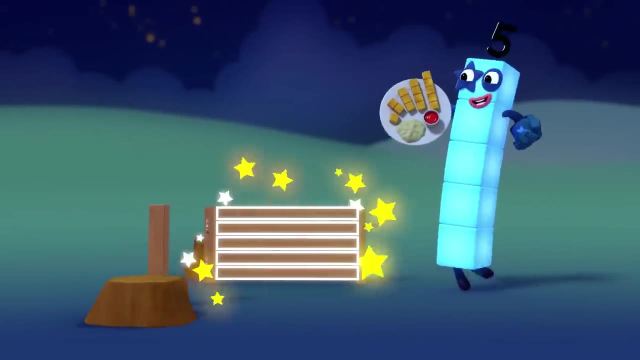 Down low too slow, High five. Ooh, I feel so alive. You know that you've arrived When you're with number five. Five fish fingers on a plate: One, two, three, four, five. Five bars on a five-bar gate: One, two, three, four, five. 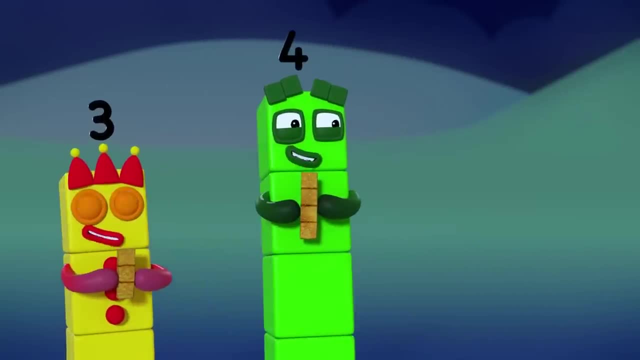 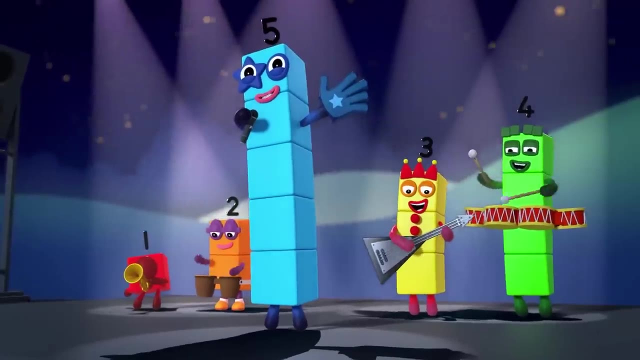 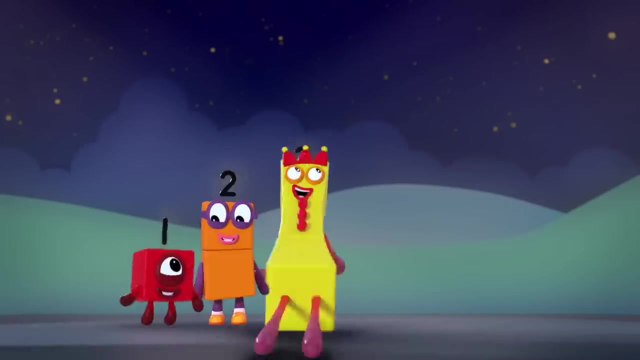 I'm fine. Ooh, I feel so alive. You know that you've arrived. When you're with number five, I'm number five And I hope you understand. Whenever you need me, I'll be there to lend a hand. Now the band is all together. The rest can join the queue. 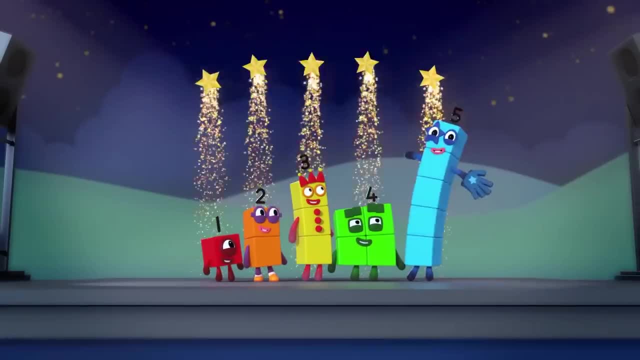 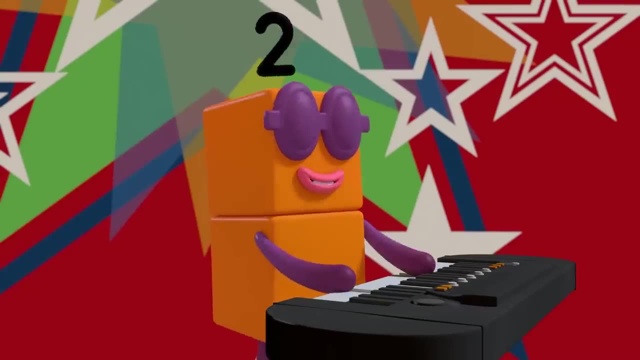 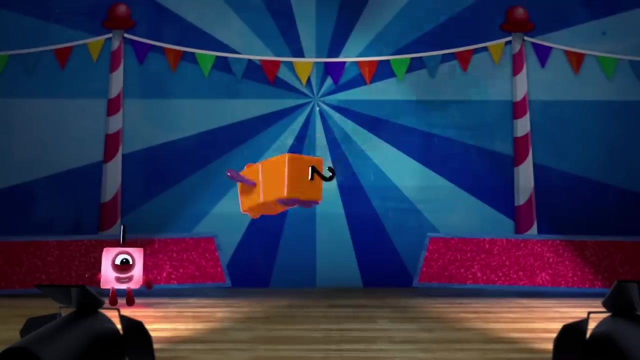 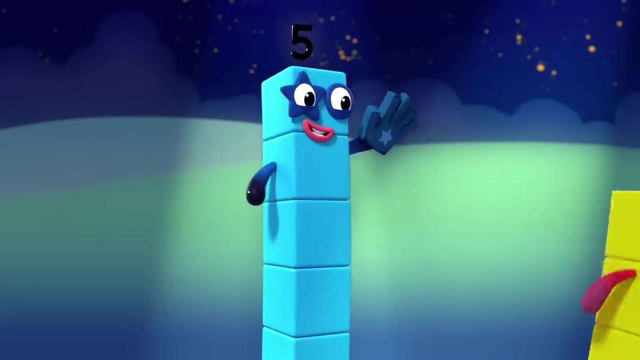 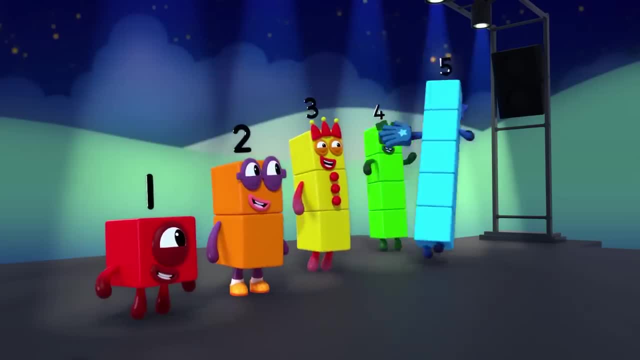 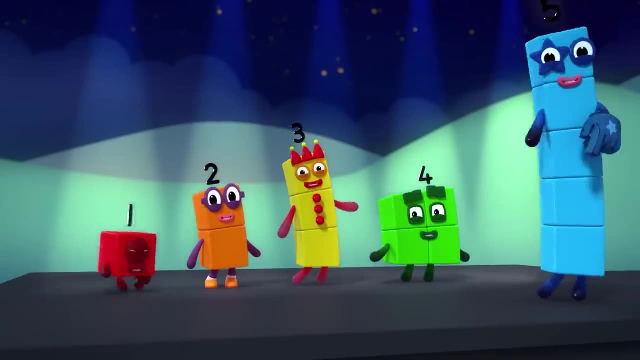 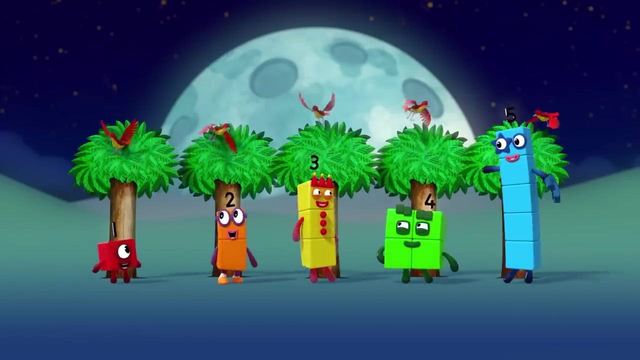 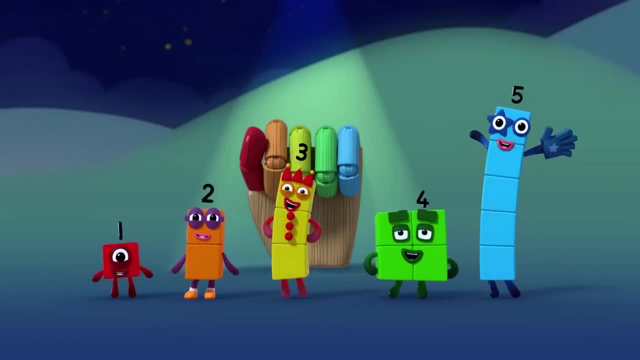 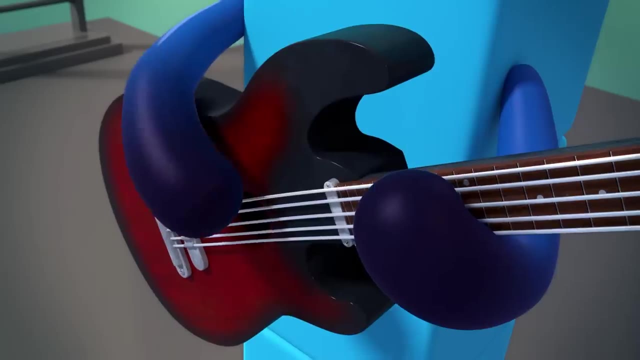 One, two, three, four, five. Everybody do the big hand-dive: One, two, three, four, five. One two, three, four, five. One, two, three, four, five, Five string, then a five string bass. 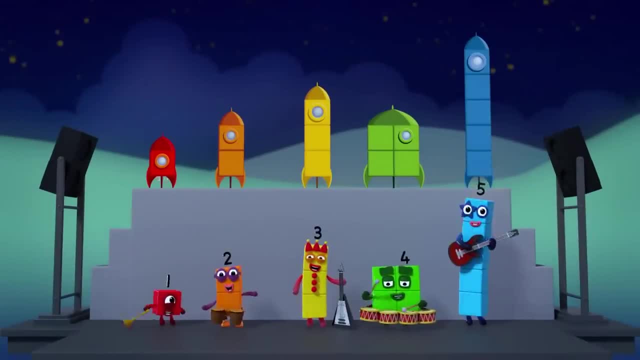 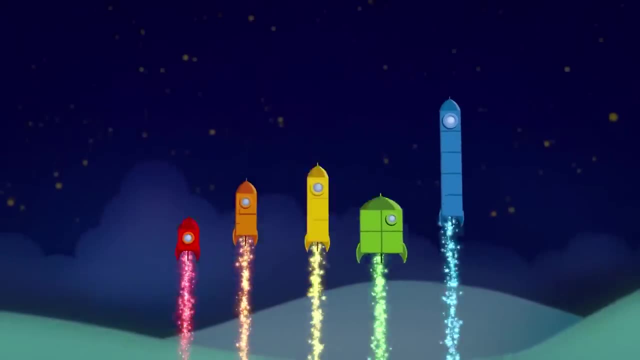 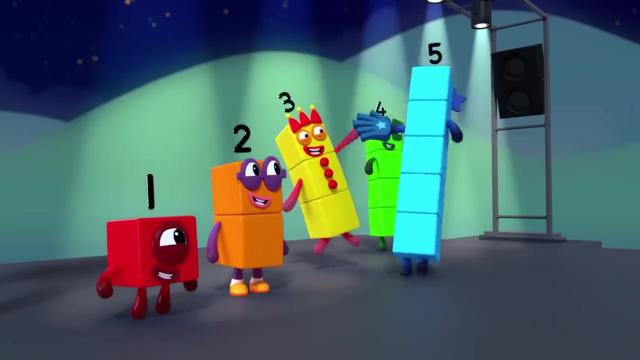 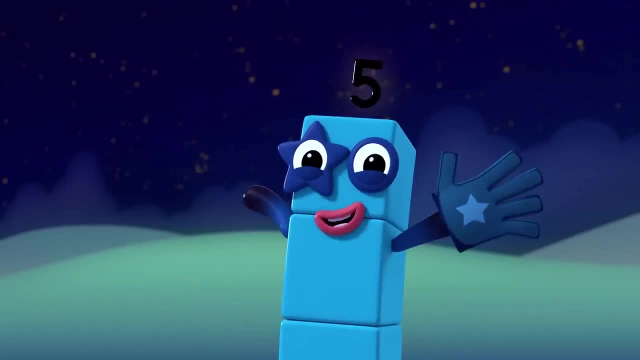 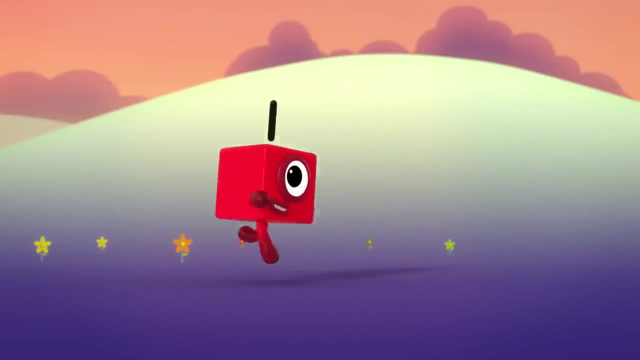 High five. Ooh, I feel so alive. You know that you've arrived. When you're with number five, I'm number one, And this is fun. I've got one block to play with And the whole of me is one. One, One, two, one, two. 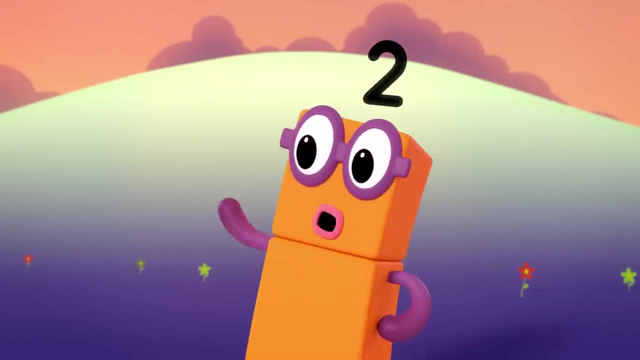 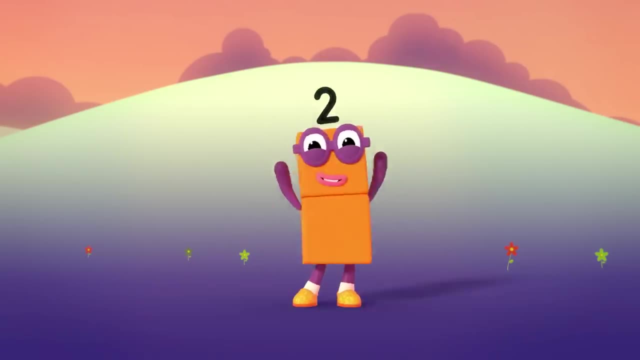 I'm number two. How do you do? I've got two blocks to play with And the whole of me is one And the whole of me is two. One, two, One is a part of me And one is a part of me And the whole of me is two. 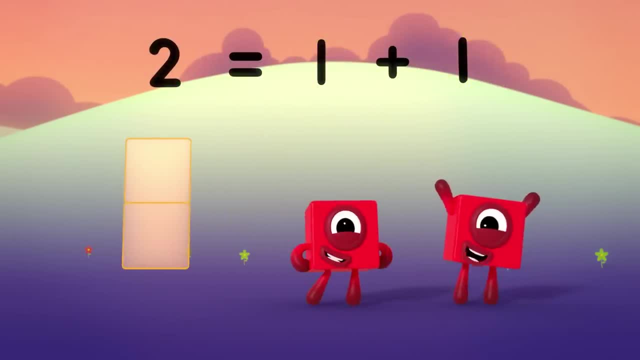 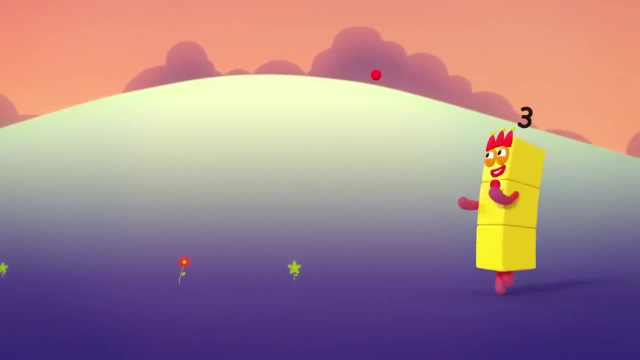 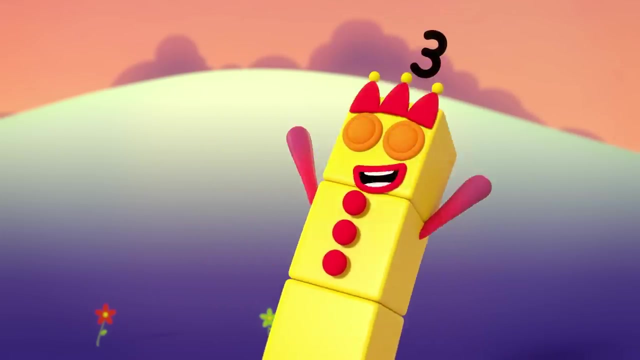 Watch. I'm one And I'm a part. I'm one And I'm a part, And the whole of me is two, One, two, three, One, two, three, One, two, three. I'm number three. Now look at me. 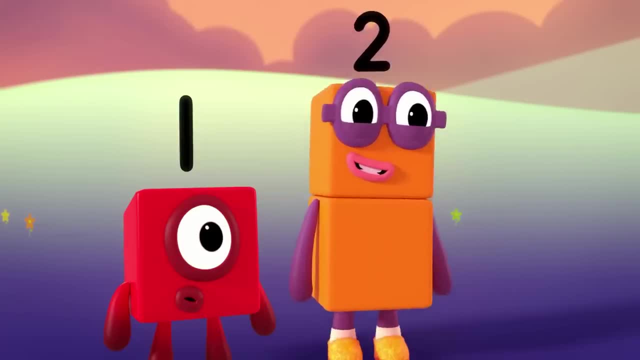 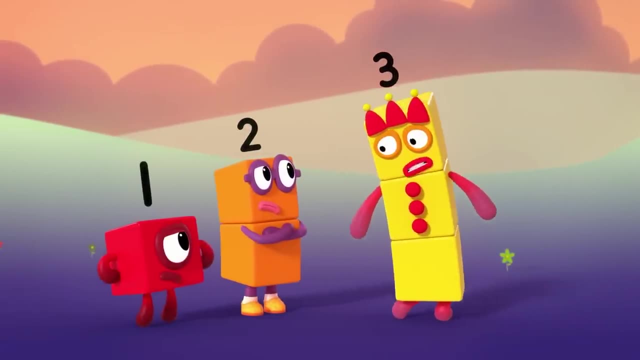 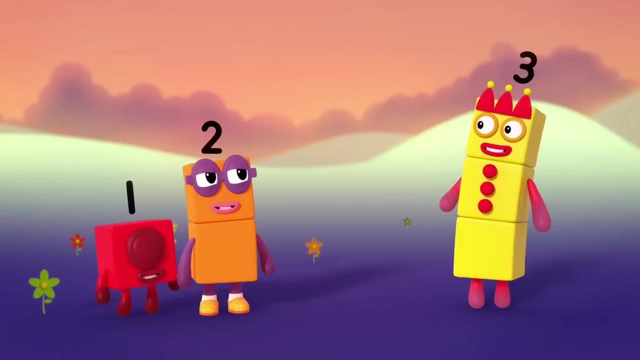 I'm the best of all the number blocks. As you can plainly see, The whole of me is amazing. The whole of me is so great. The whole of me is Sorry. Three, Try again. Okay, I'm number three. Yes, look at me, I'm the best of all the number blocks. 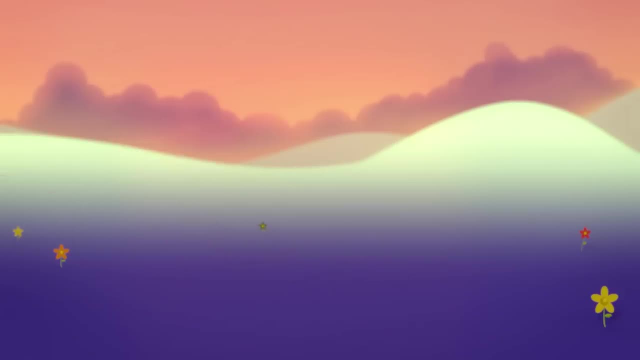 Oh, you can't do it like that. You can't do it like that, You can't. you're quite as good as you try. Aww, one more time. I'm number three. Now look at me. I've got three blocks to play with. 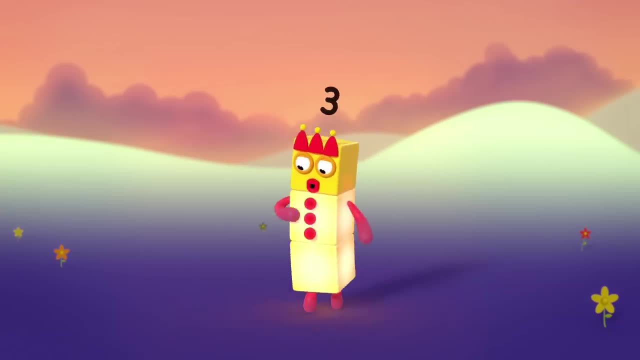 And the whole of me is three. One, two, three. One is a part of me And two is a part of me, And the whole of me is three. Watch, I'm two And I'm a part. I'm one And I'm a part. 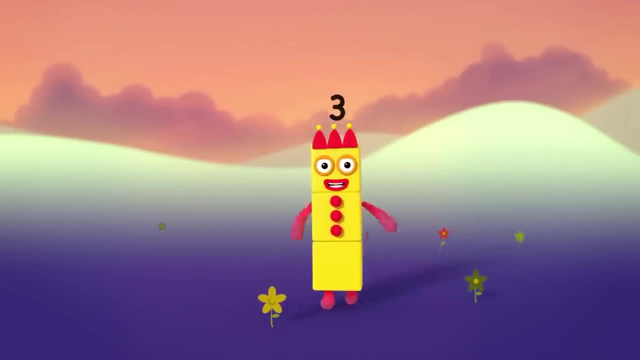 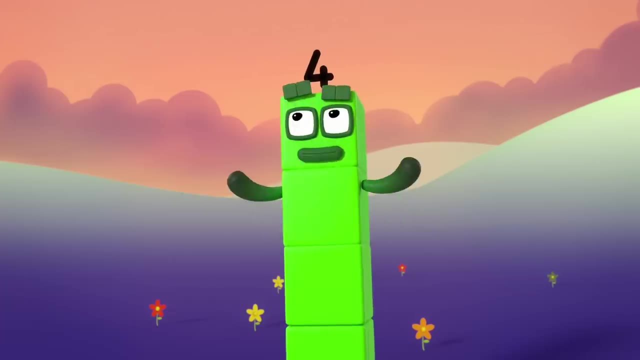 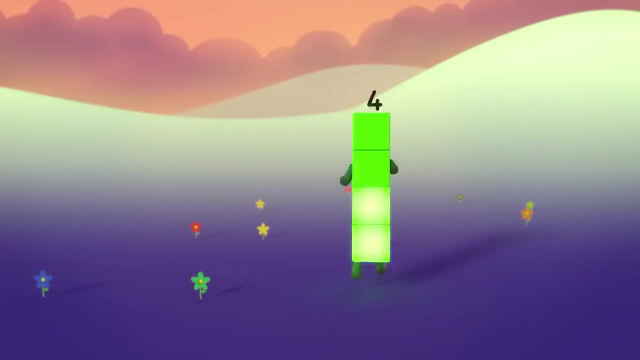 And the whole of me is three, One, two, three. I'm number four And I am sure that I've got four blocks to play with And the whole of me is four. One, two, three, four. One is a part of me. 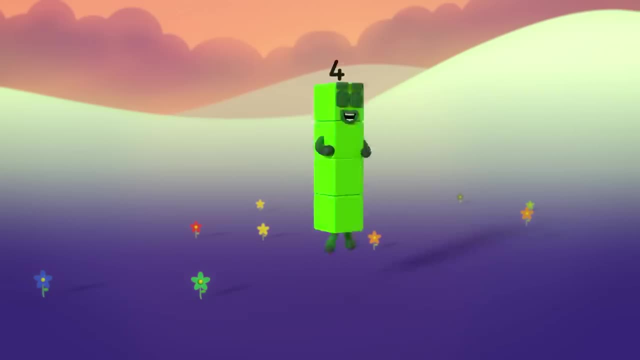 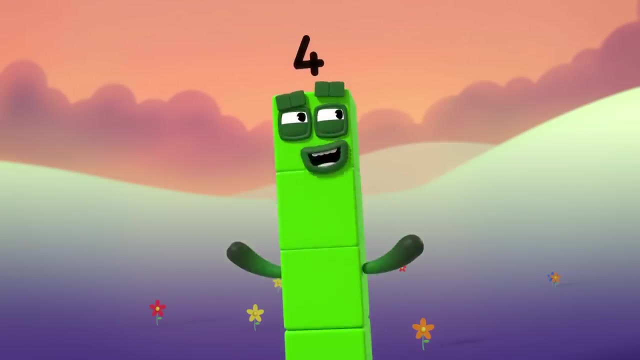 And three is a part of me And the whole of me is four. What I'm three and I'm a part. I'm one and I'm a part, And the whole of me is four. Now, here is something more that's different from before. 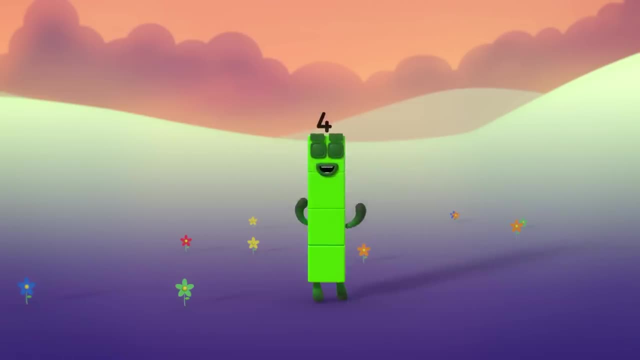 Two is a part of me, And two is a part of me And the whole of me is four. What I'm two and I'm a part. I'm two and I'm a part, And the whole of me is four. 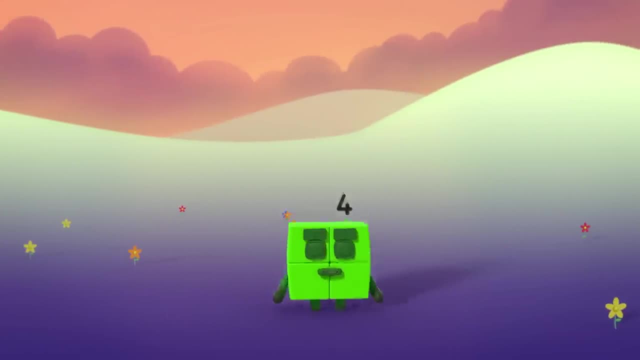 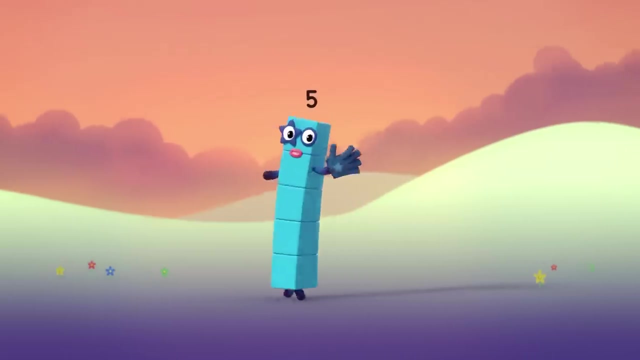 I'm a square. look Four sides, four corners. I'm number five. I am alive, I've got five blocks to play with And the whole of me is five. One, two, three, four. five One is a part of me. 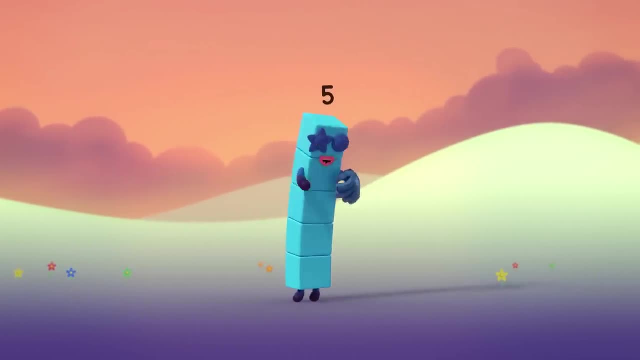 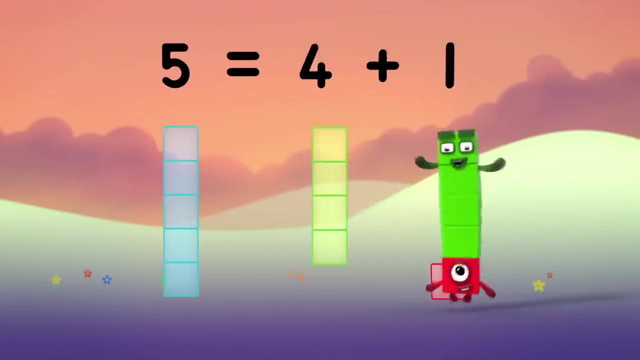 And four is a part of me And the whole of me is five. What I'm four and I'm a part. I'm one and I'm a part, And the whole of me is four And the whole of me is five. 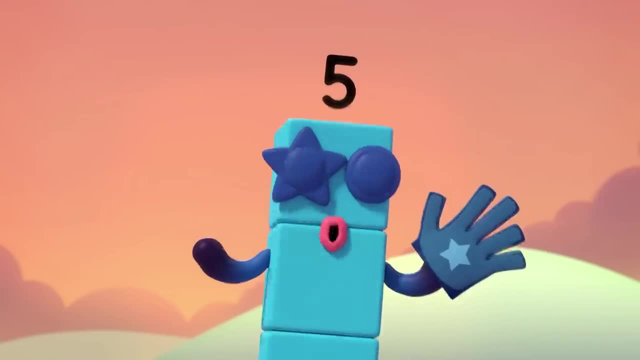 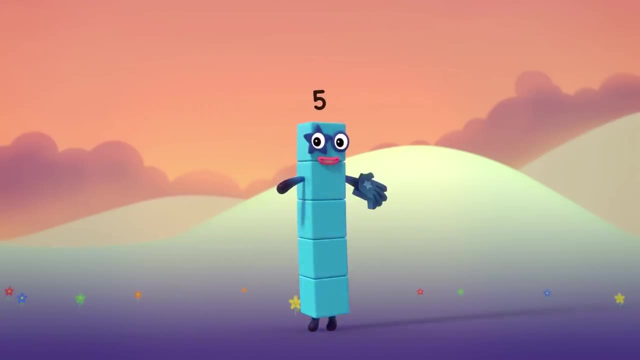 And the whole of me is five And the whole of me is five. But now I feel alive. going into overdrive, Two is a part of me And three is a part of me, And the whole of me is five. One and three and I'm a part. 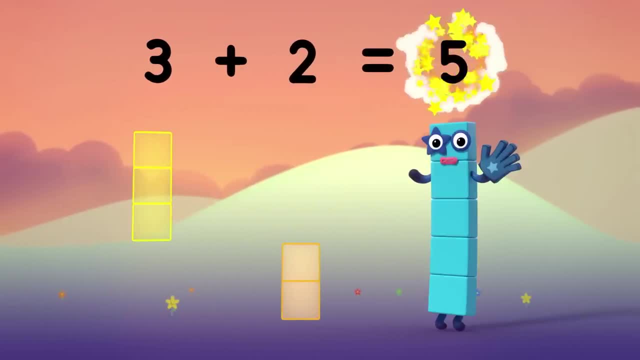 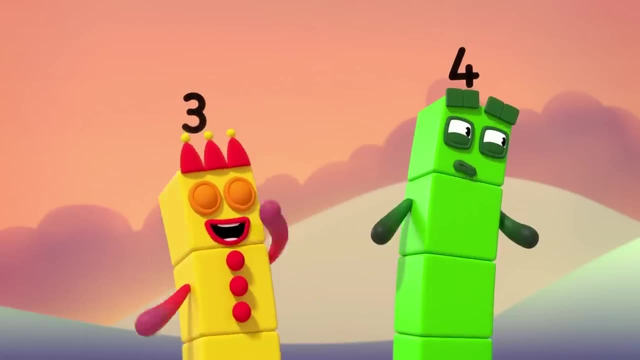 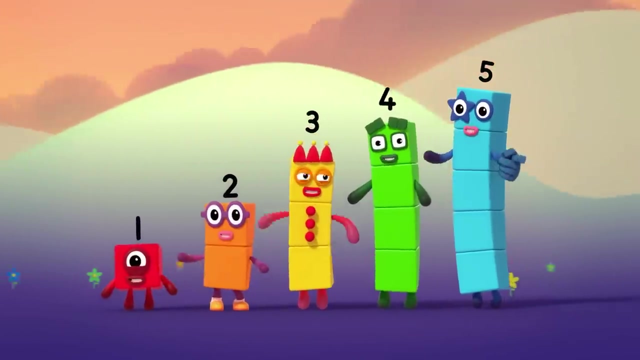 I'm two and I'm a part, And the whole of me is five High five. Making friends is easy when you can come apart. Splitting up is not so hard, it won't break your heart. So when we fall to pieces, we have lost control. 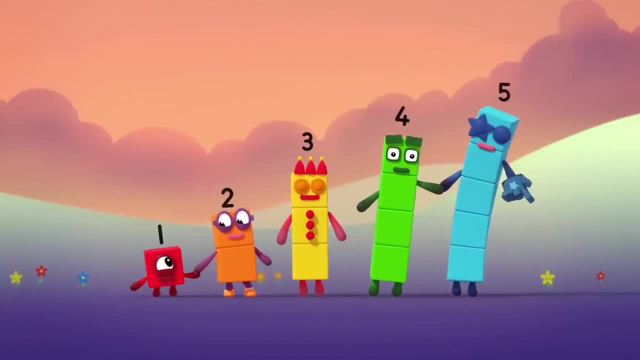 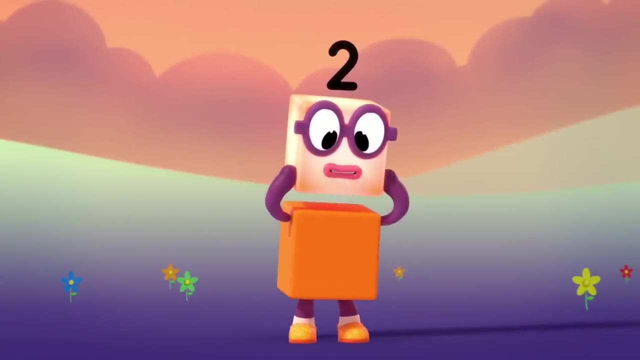 A whole is made of all its parts and the parts they make a whole. Just remember that One is a part of me and one is a part of me. One is a part of me and two is a part of me. 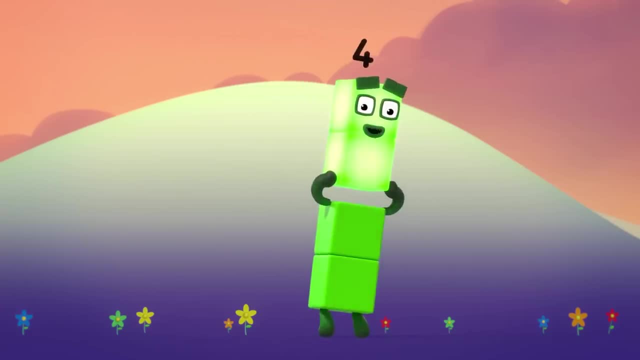 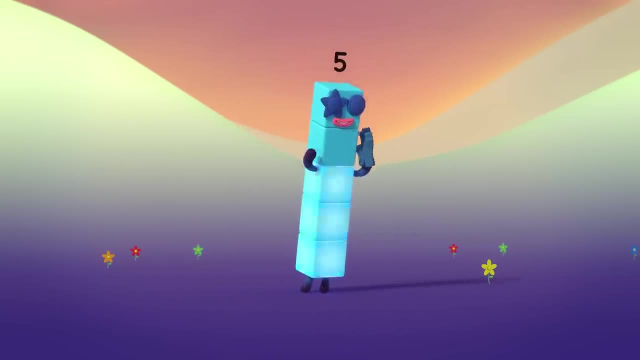 One is a part of me and three is a part of me. Two is a part of me and two is a part of me. One is a part of me and four is a part of me. Two is a part of me and three is a part of me. 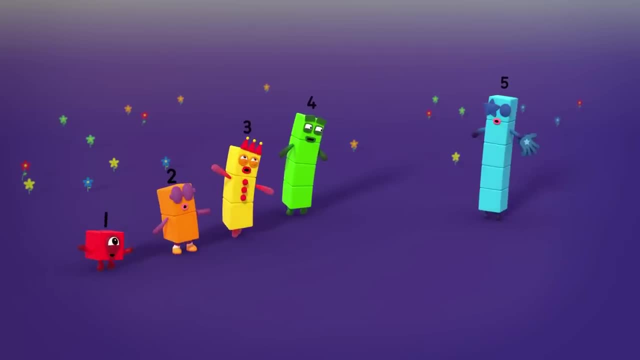 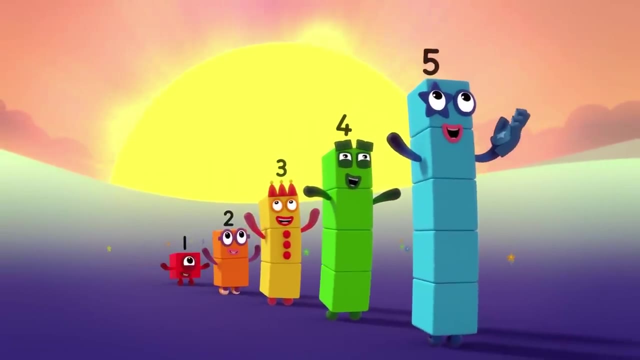 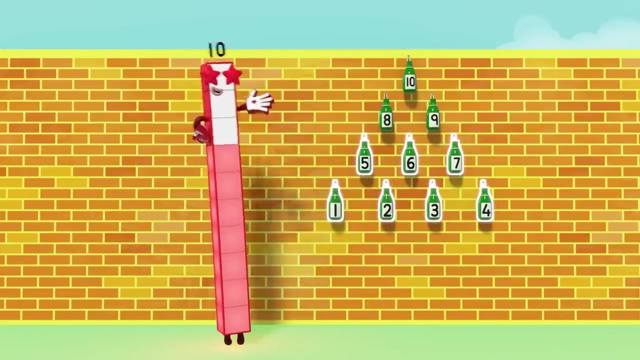 One is a part of me and four is a part of me, And the whole of me is one, two, three, four, five. One, two, three, four, five, six, seven, eight, nine, ten. 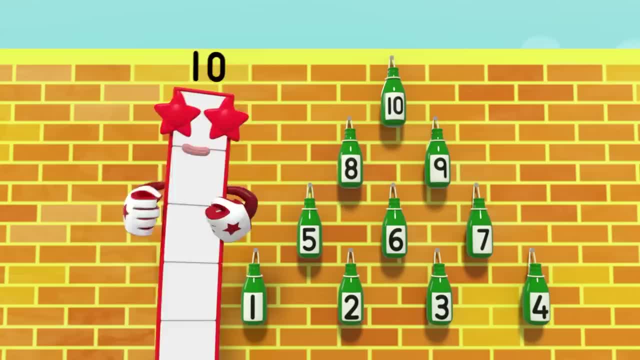 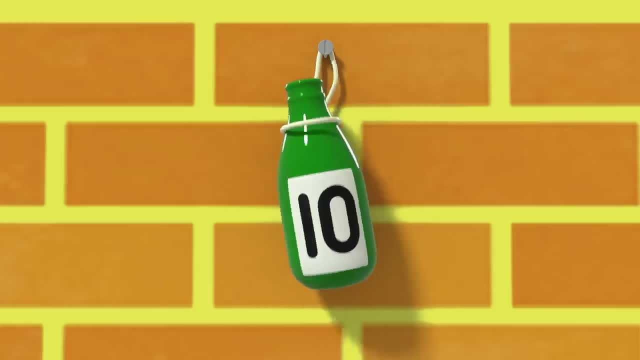 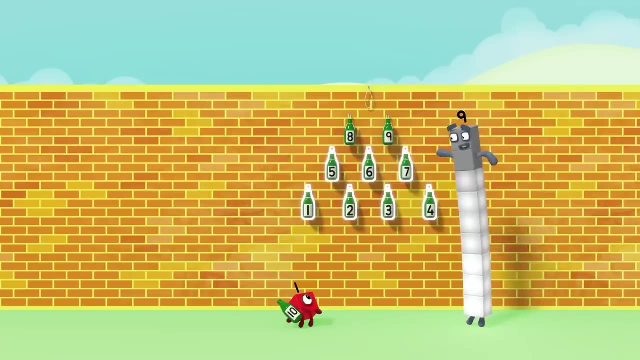 Ten green bottles. Ten green bottles hanging on the wall, Ten green bottles hanging on the wall, But if one green bottle should accidentally fall, There'll be one, two, three, four, five, six, seven, eight, nine, Nine green bottles hanging on the wall. 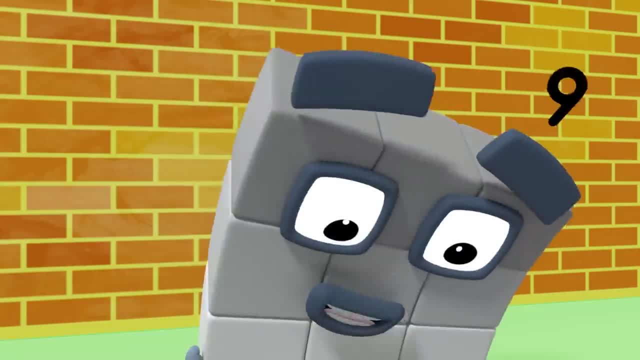 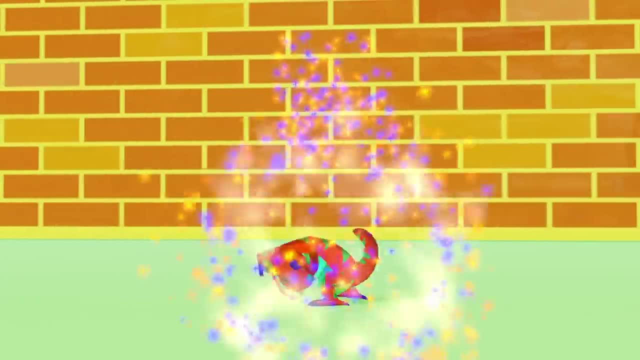 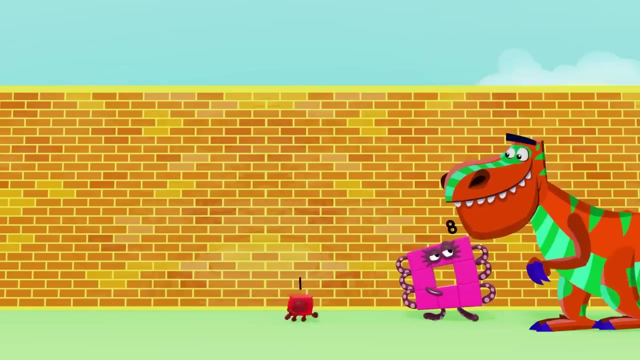 Better move these nine before they fall. They're not safe up there. Nine green bottles safely on the floor. Nine green bottles safely on the floor. Oh, oh, ah, ah, ah, achoo. But if one green bottle becomes a dinosaur, 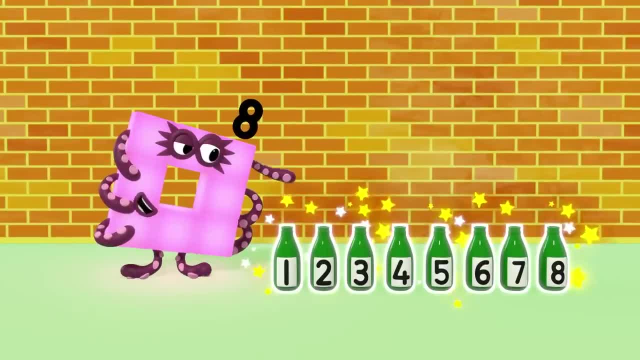 There'll be one, two, three, four, five, six, seven, eight, Eight green bottles. not safe on the floor, Octoblock hide. One, two, three, four, five, six, seven, eight hide. 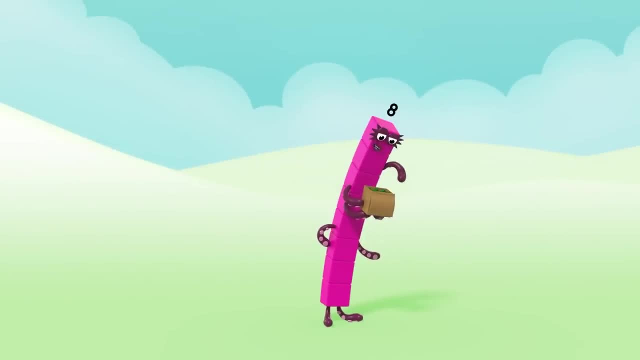 Eight green bottles hiding in a box. Eight green bottles hiding in a box. But if one green bottle is stolen by a fox, Hey, There'll be one, two, three, four, five, six, seven, Seven green bottles hiding in a box. 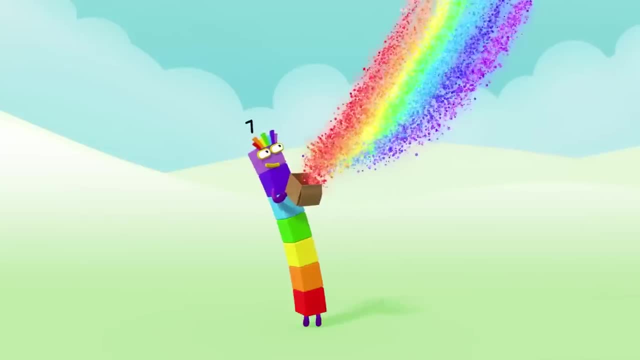 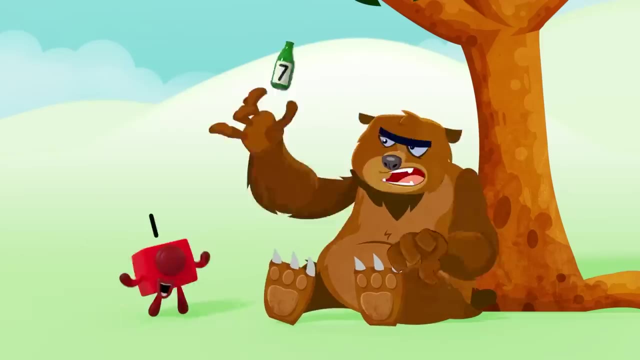 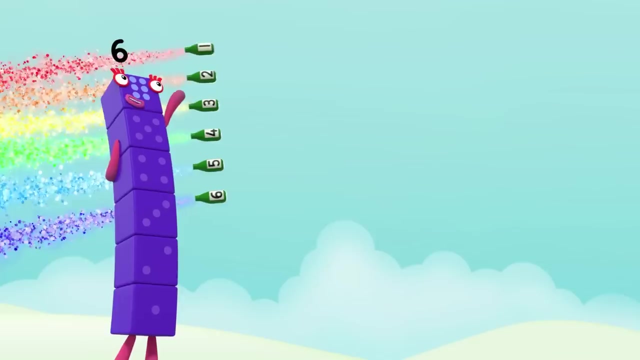 That was lucky. Ooh, Seven green bottles flying through the air. Seven green bottles flying through the air. But if one green bottle should wake, a grizzly bear, What I mean? hug a teddy bear. Phew, There'll be one, two, three, four, five, six. 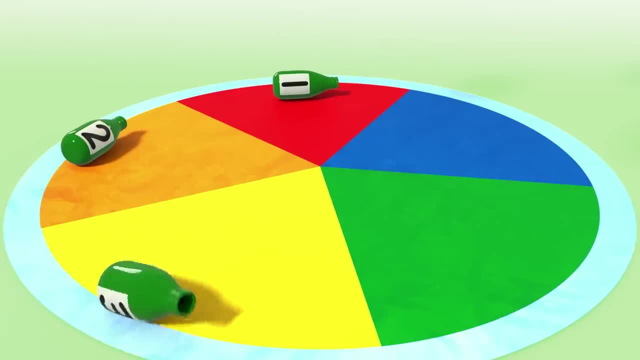 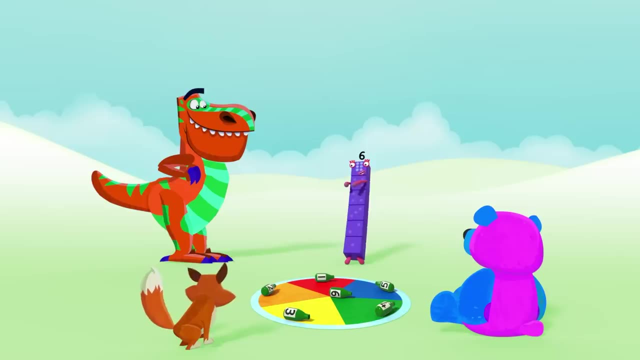 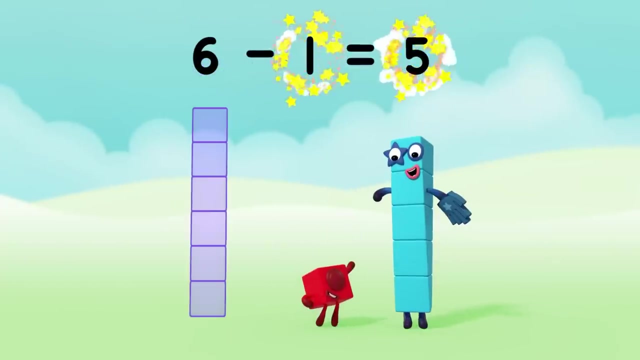 Six green bottles falling through the air. Six is my name. Let's play a game, And this game goes like this: Six green bottles lying on the ground, Six green bottles lying on the ground, And if one green bottle spins around, Whoa. 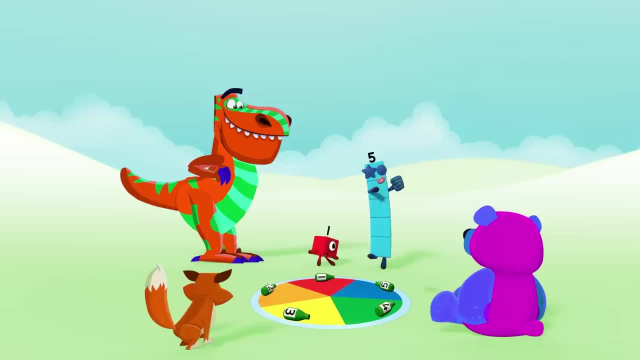 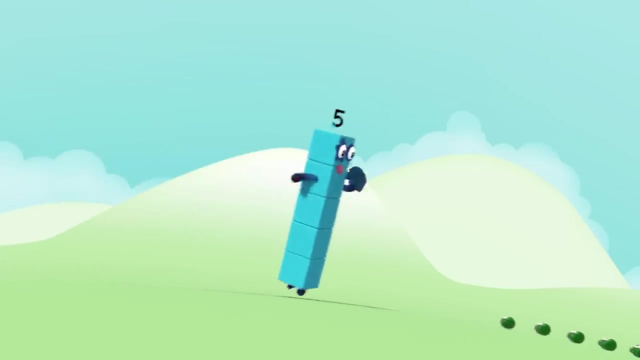 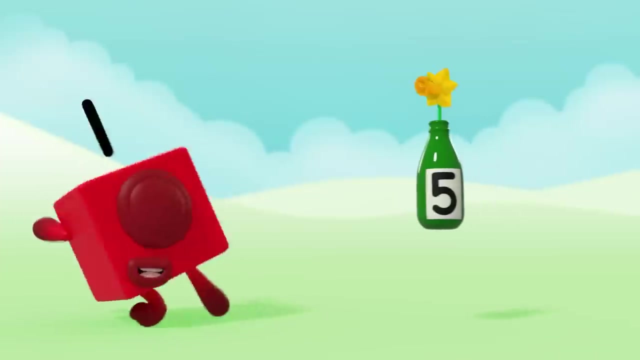 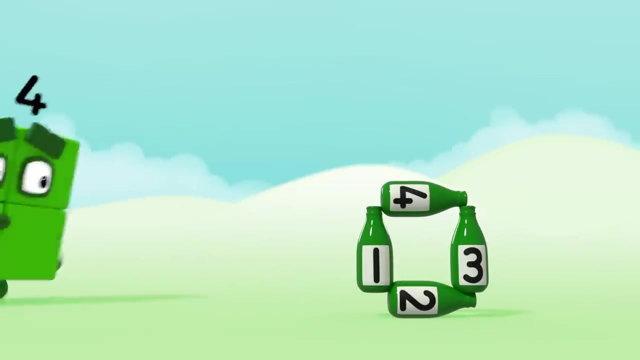 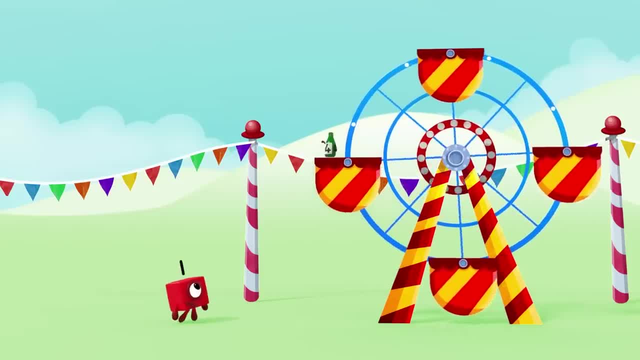 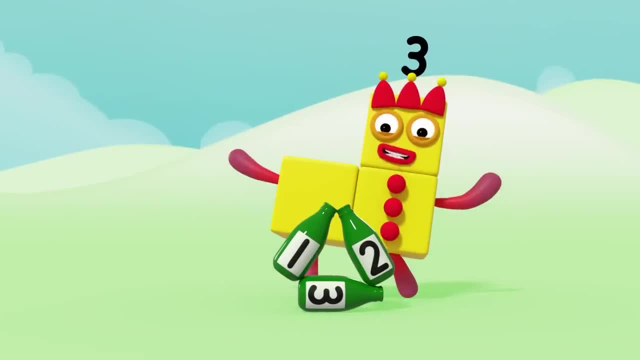 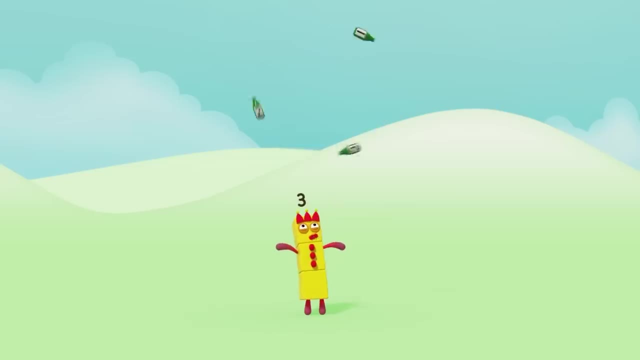 There'll be one, two, three, three green bottles standing in a triangle. One, two, three, three green bottles spinning in the sky. Three green bottles spinning in the sky, But just one green bottle should drop its wings and fly. 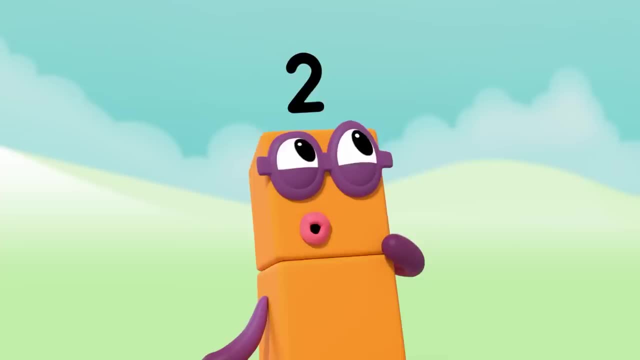 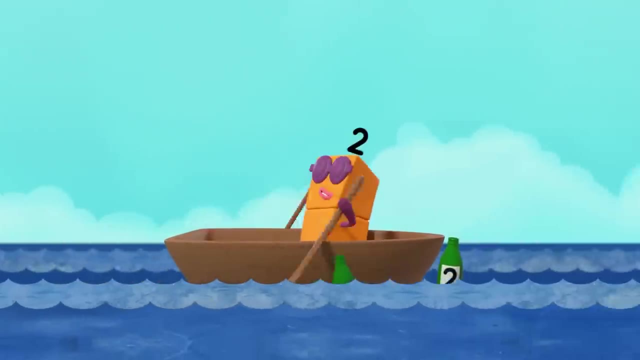 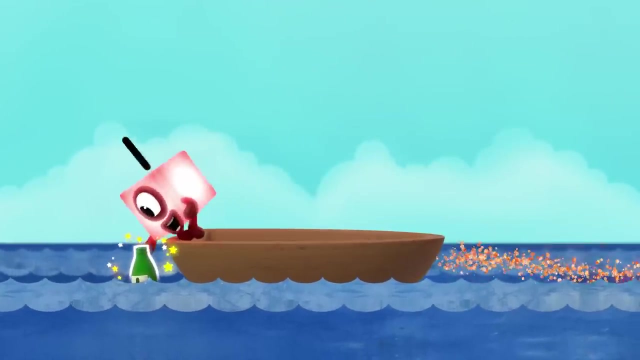 There'll be one, two, three green bottles spinning in the sky. Come back Two green bottles floating out to sea, Two green bottles floating out to sea. But if one green bottle should learn to water sea, There'll be one, one green bottle floating out to sea. 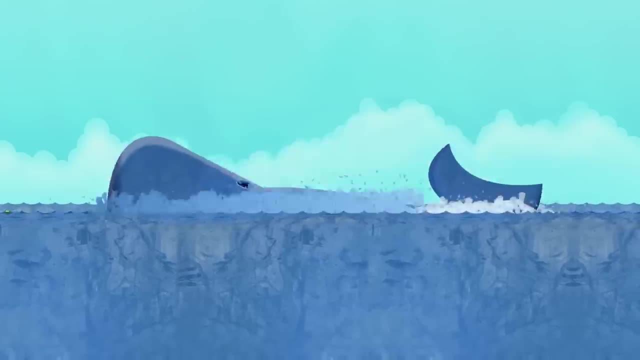 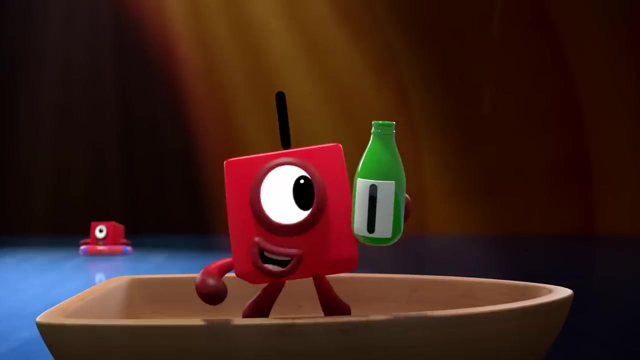 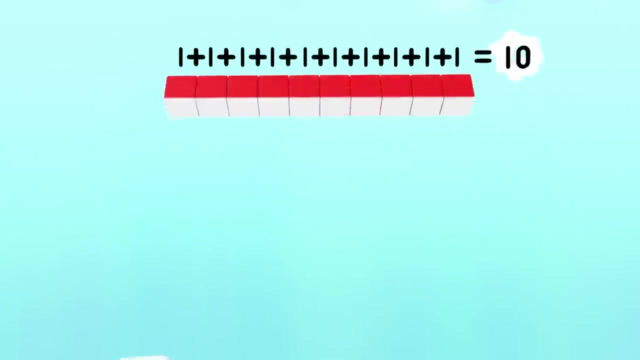 One green bottle swallowed by a whale. One green bottle swallowed by a whale. But if that green bottle should grow a tickly tail, There'll be no green bottle swallowed by a whale. Ten green bottles hanging on a wall, Safely on the floor, hiding in a box. 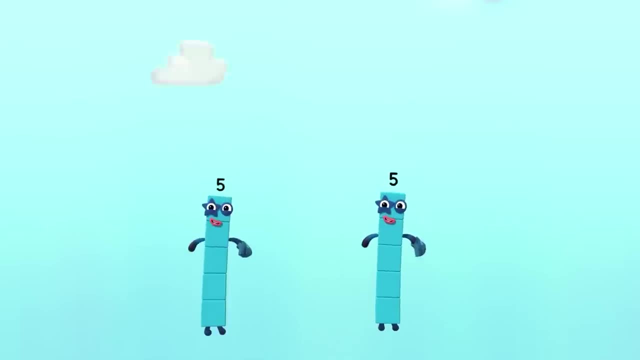 Flying through the air, lying on the ground, Ten green bottles rolling down a hill, Standing in a square, spinning in the sky, Floating out to sea swallowed by a whale. But if one green bottle should accidentally fall, Become a dinosaur, wake, a grizzly bear. 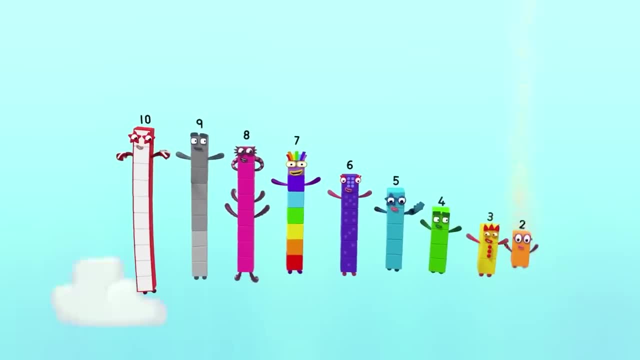 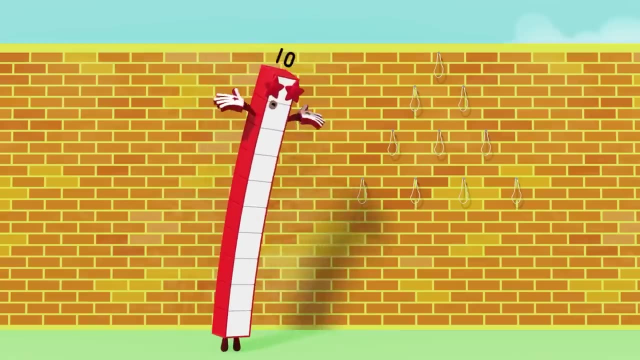 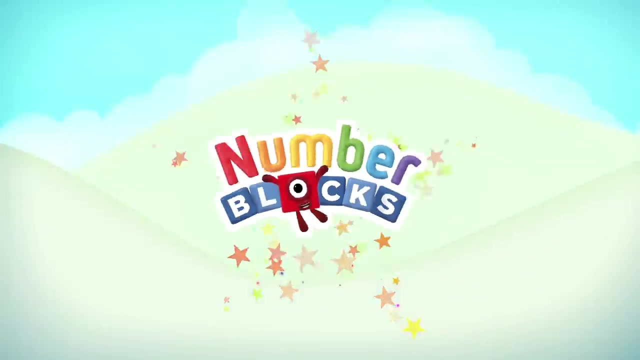 Step in a round up a tube, Flap its wings and fly. Learn to water ski, Grow a tickly tail. There'll be nine, eight, seven, six, five, four, three, two, one. No green bottles hanging on the wall. Number Blobs. 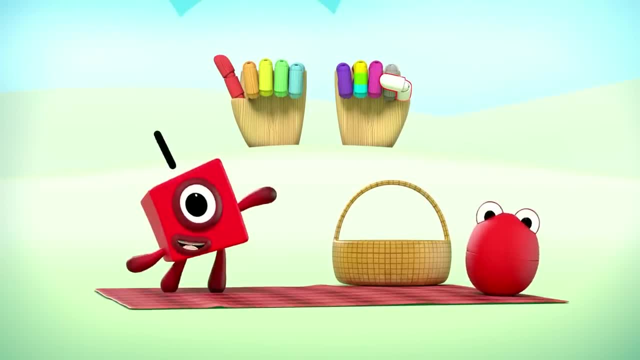 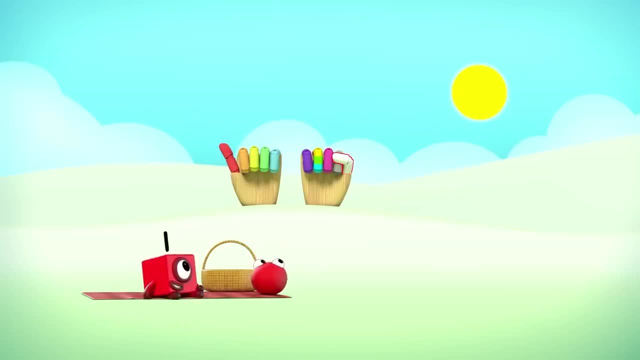 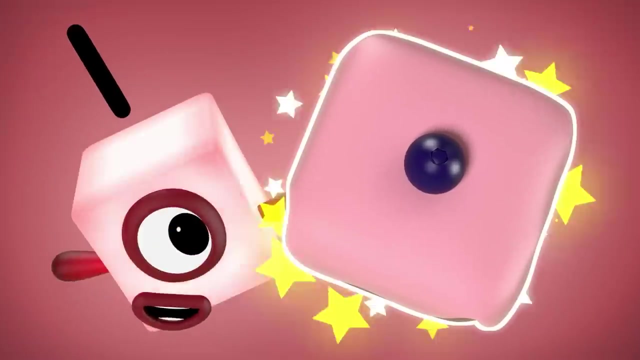 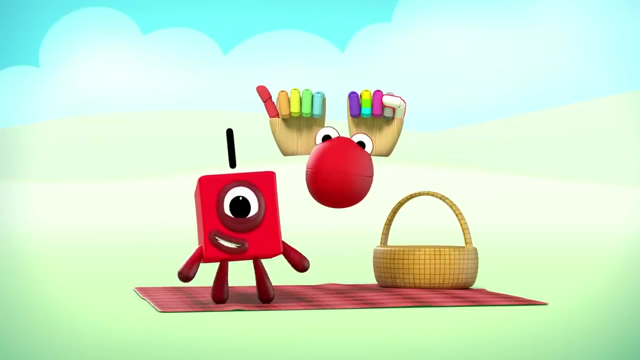 One, two, one, two, three, four. One number blob and me Counting everything we see, Sharing a bun, Sitting in the sun, Whistling a happy melody: One number blob and me. One one bun, One one sun. One number blob and me. 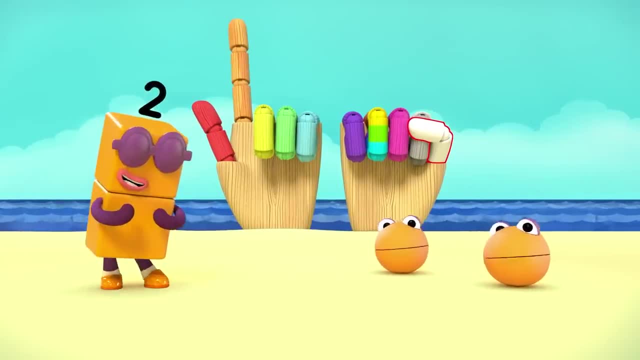 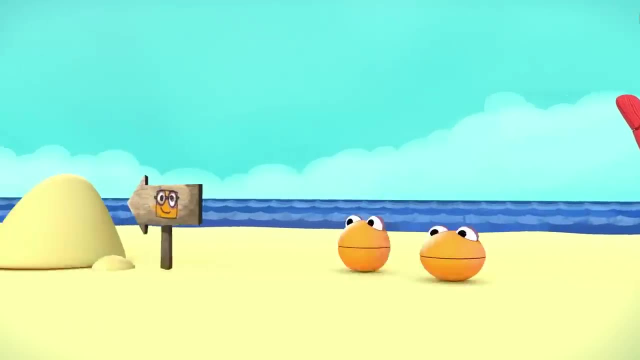 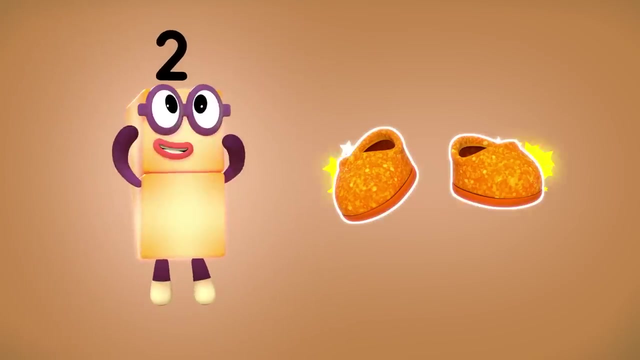 Two number blobs and me Counting everything we see Taking off our shoes. Lucky bought our clothes Whistling a happy melody. Two number blobs And me One, two, two shoes. Two number blobs and me One, two, two shoes. One, two, two clothes. 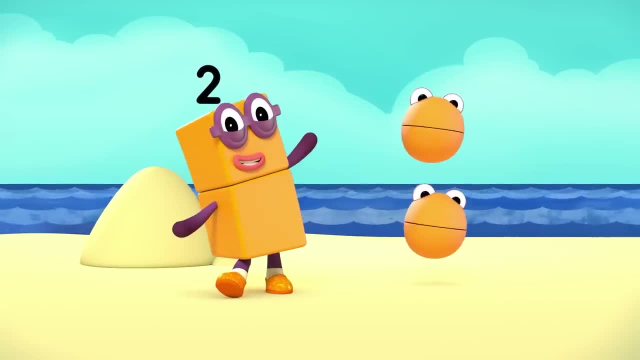 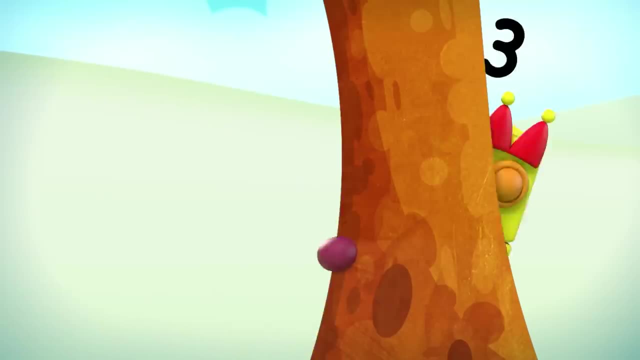 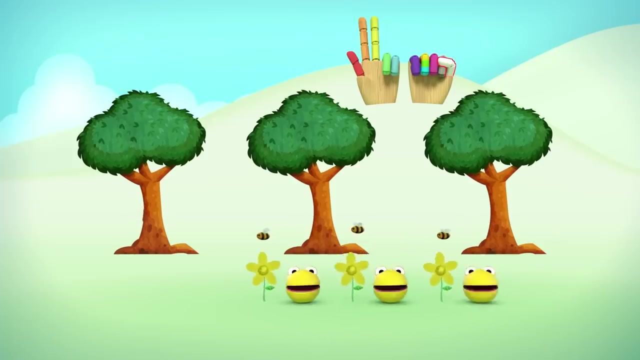 Two number blobs and me. Three number blobs and me Counting everything we see Hiding in the trees, Whistling a happy melody. Three number blobs and me. One, two, three, Three trees. One, two, three, Three bees. One, two, three, Three bees. 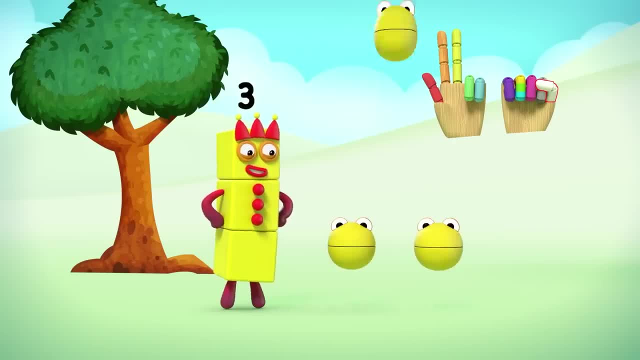 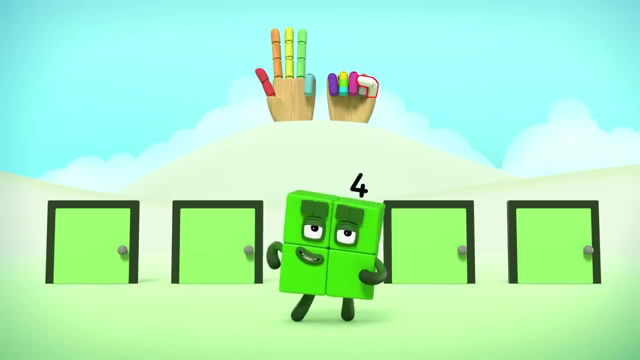 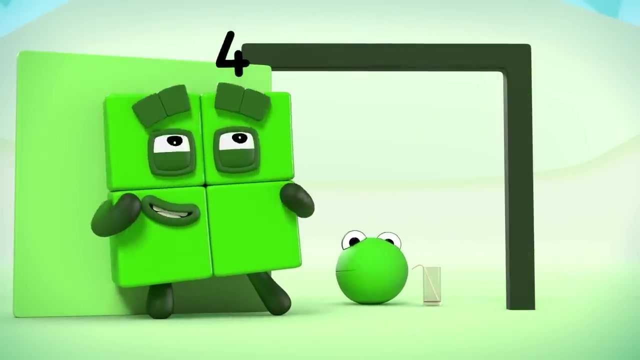 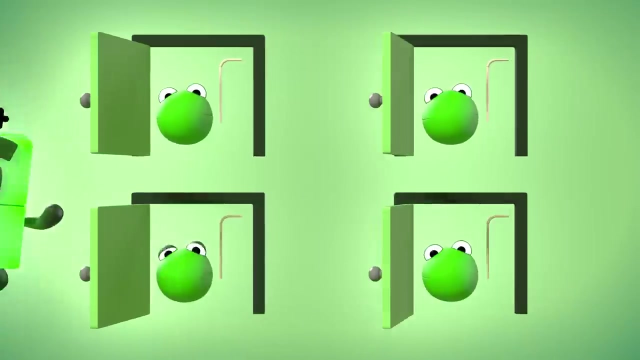 Three bees. three number blobs And me. Four number blobs and me Counting everything we see Opening the door, surfing through a storm, Whistling, a happy melody. Four number blobs and me. One, two, three, four, four doors. One, two, three, four, four stars. 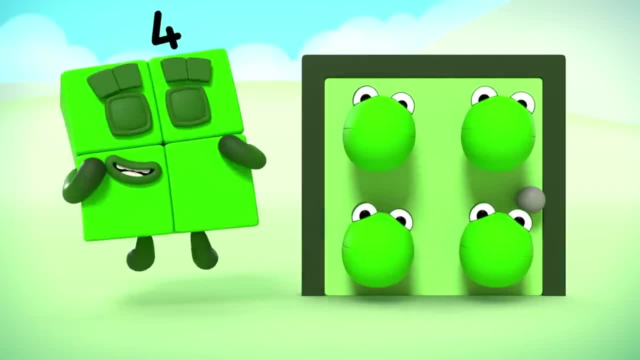 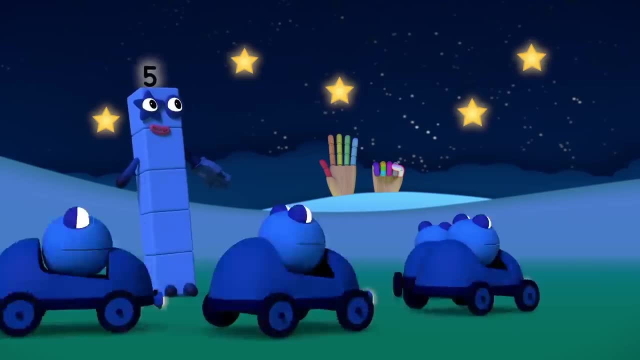 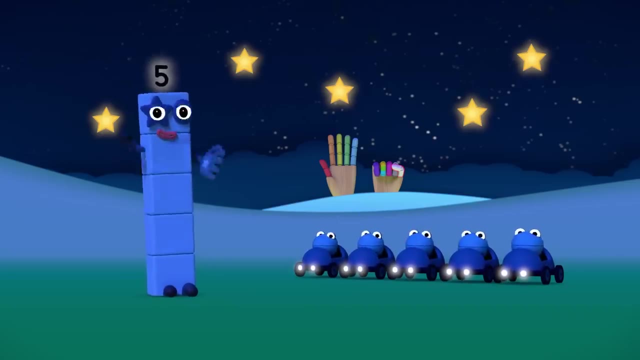 Four number blobs and me. Five number blobs and me Counting everything we see, Gazing at the stars, parking, all the cars Whistling, a happy melody. Five number blobs and me. One, two, three, four, five, five stars. One, two, three, four, five, five cars. 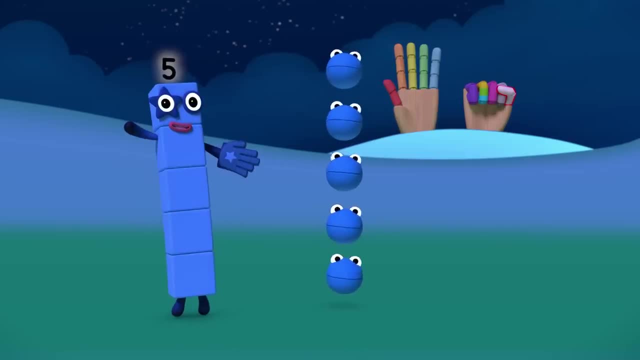 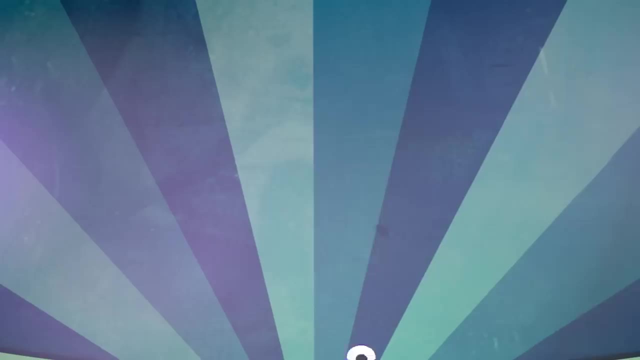 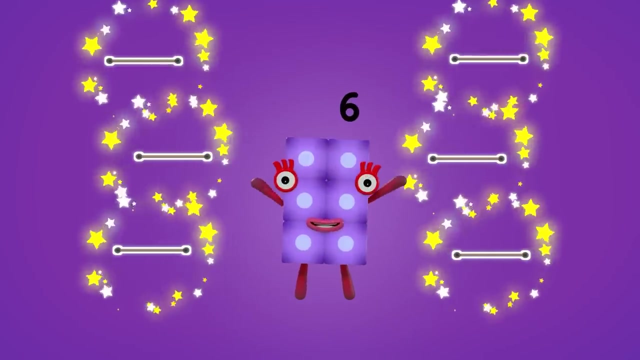 Five number blobs and me. Six number blobs and me, Counting everything we see Picking up a stick showing off a trick. Six number blobs and me. One, two, three, four, five, six, Six sticks. one, two, three, four, five, six. 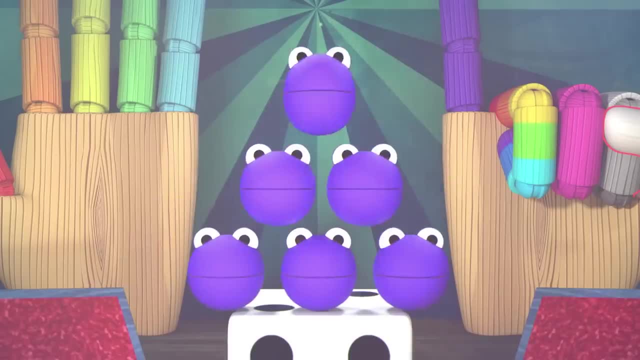 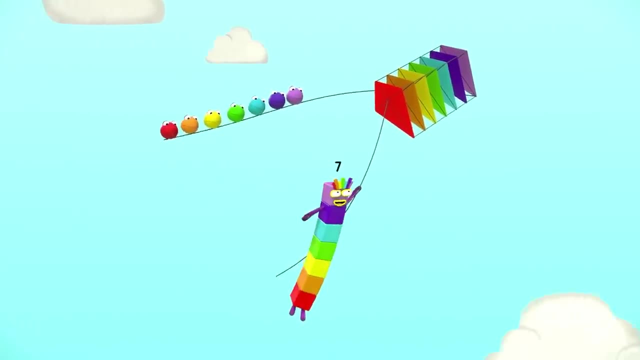 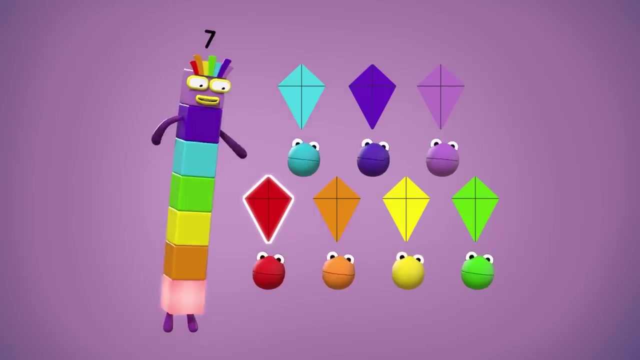 Six tricks. six number blobs And me, Seven number blobs and me Counting everything we see Flying a kite, three, four kite Turning on the lights, three, four kite Rainbow lights. seven number blobs And me, One, two, three, four, five, six, seven. 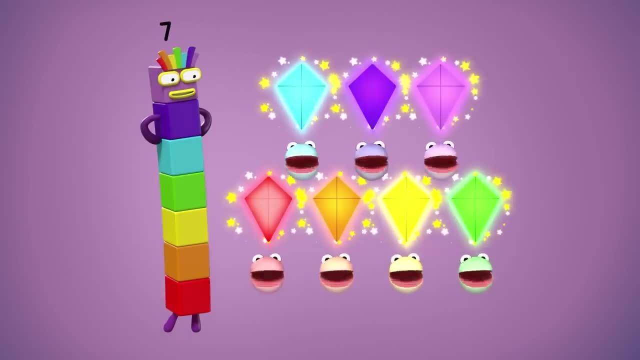 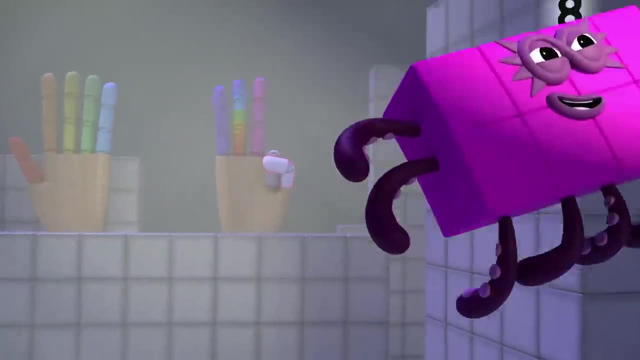 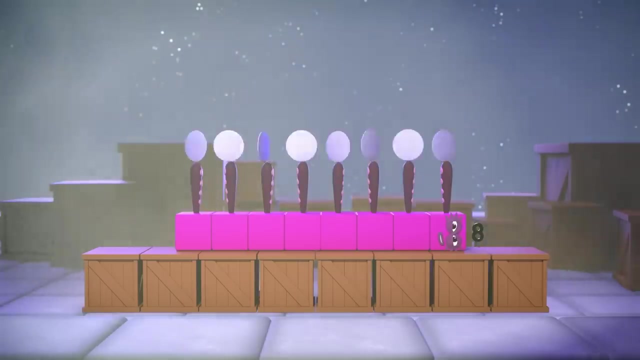 Seven kites: one, two, three, four, five, six, seven, Seven lights, seven number blobs And me, Eight number blobs and me Counting everything we see, Spinning all the plates off the block. spin, Lifting all the crates, number blobs, lift. 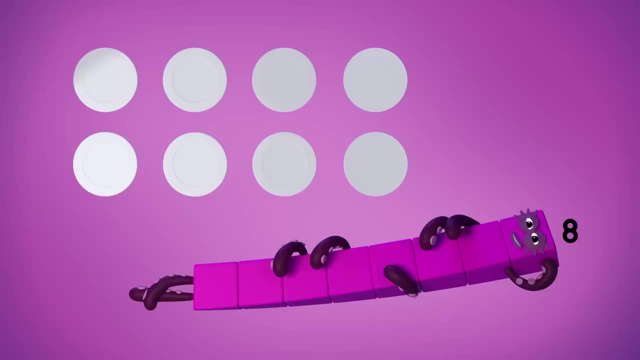 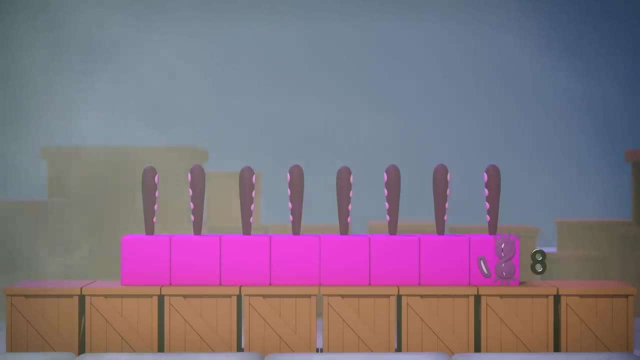 Eight number blobs and me. One, two, three, four, five, six, seven, eight Eight plates. one, two, three, four, five, six, seven, eight, Eight plates. eight number blobs And me. Nine number blobs and me. 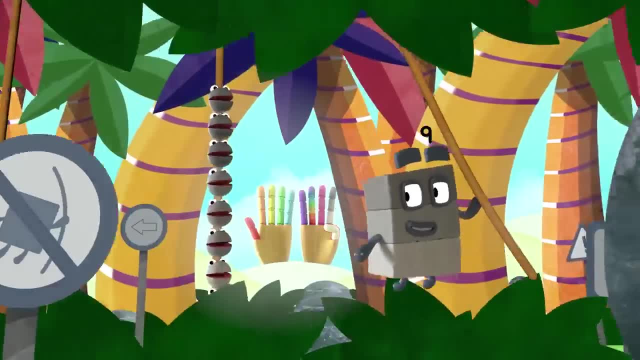 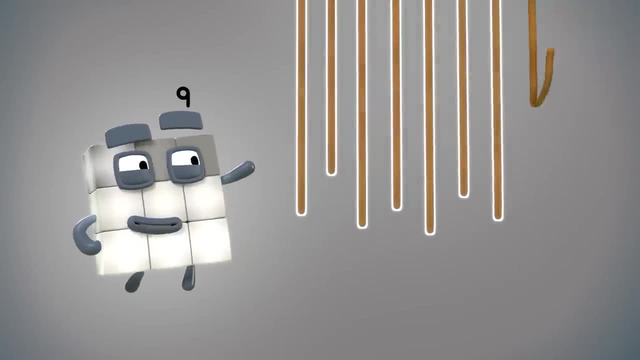 Counting everything we see, Swinging through the vines, Ignoring all the signs. Nine number blobs and me: One, two, three, four, five, six, seven, eight, nine, Nine vines: One, two, three, four, five, six, seven, eight, nine. 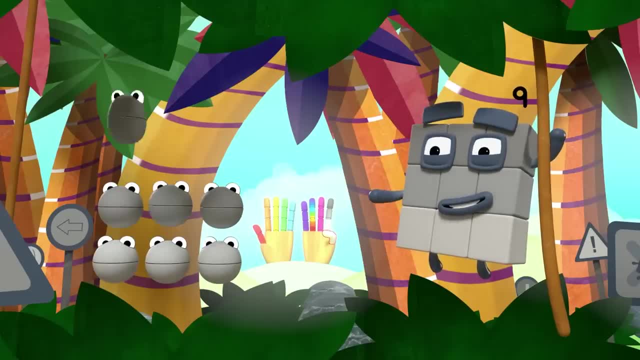 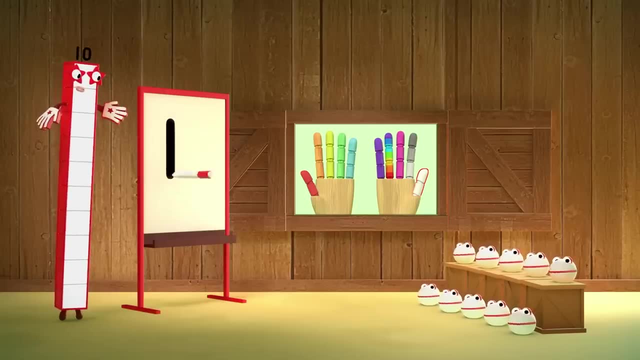 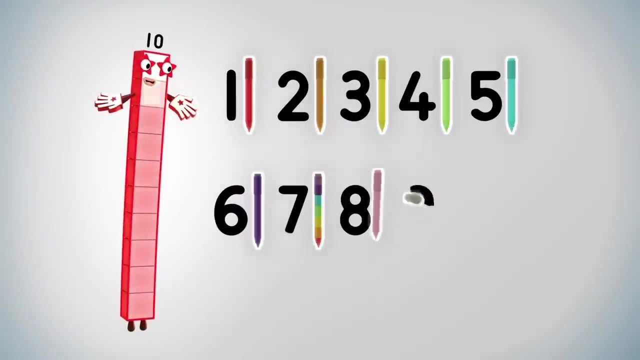 Nine signs, Nine number blobs, Eight spinning blades, Eight heavy crates And me. Ten number blobs and me Counting everything we see Writing with a pen Plop like a hen. T-t-t-t-ten number blobs And me: One, two, three, four, five, six, seven, eight, nine, ten. 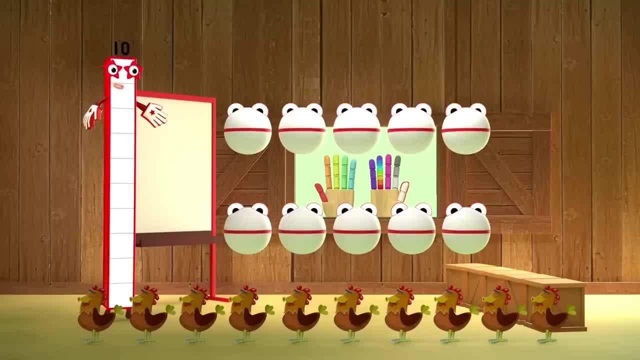 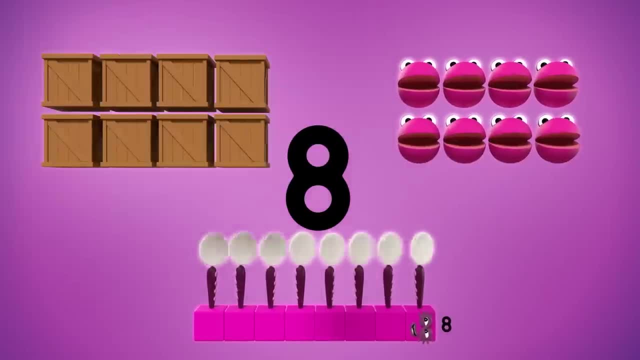 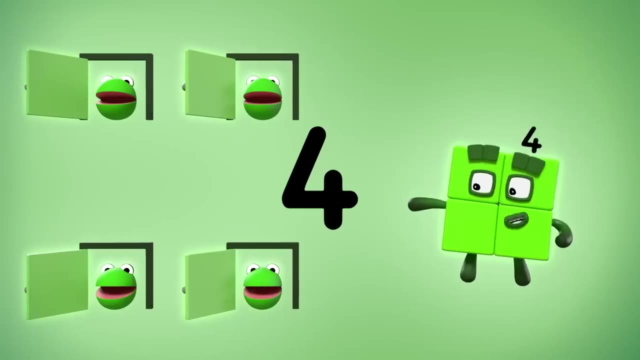 Ten pens. One, two, three, four, five, six, seven, eight, nine, ten, Ten pens. Ten number blobs, Seven floating kites, seven rainbow lights, Six wooden sticks, six clever tricks, Five shooting stars, five motor cars, Four open doors, four bendy straws. 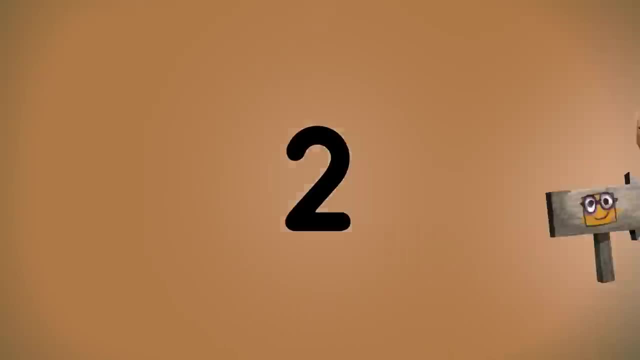 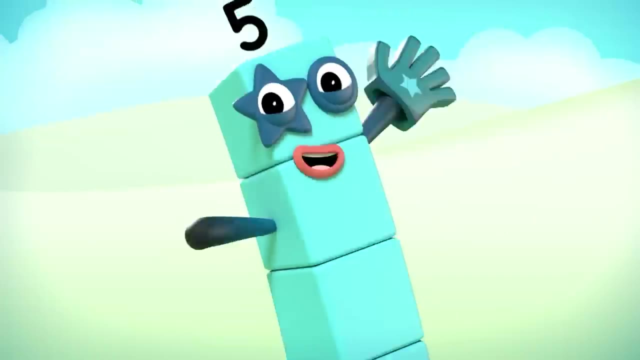 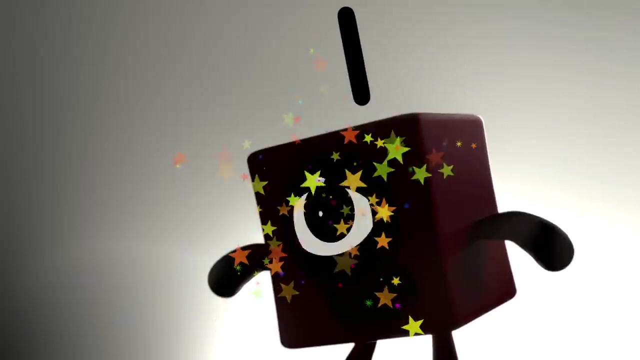 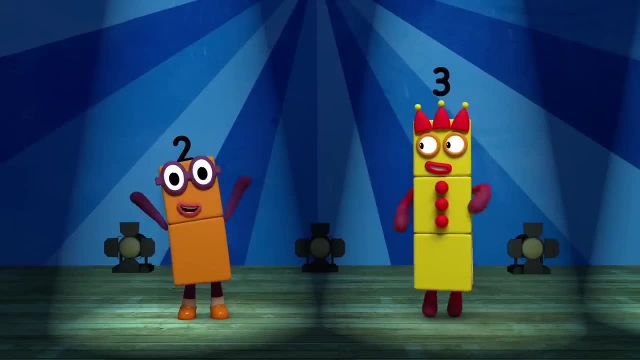 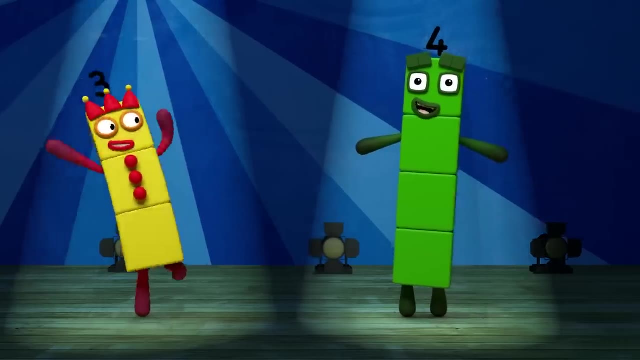 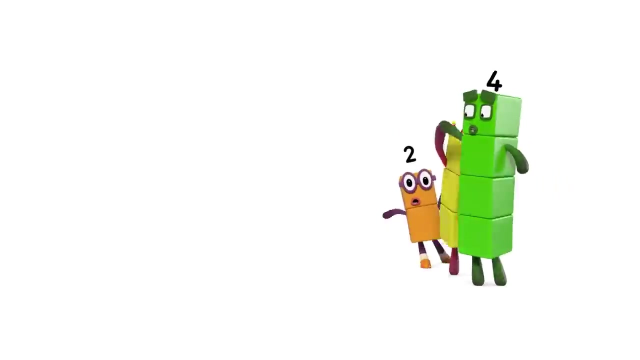 Three is bigger than two. I can hide behind you. Four is bigger than three. Three can hide behind me. Peek-a-boo, I'm hiding behind you Cause I'm bigger than you. no one will find you. Where have they gone? Go on, Give us a clue. can you see me? 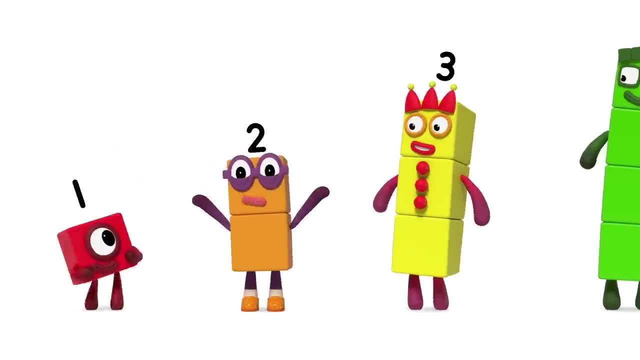 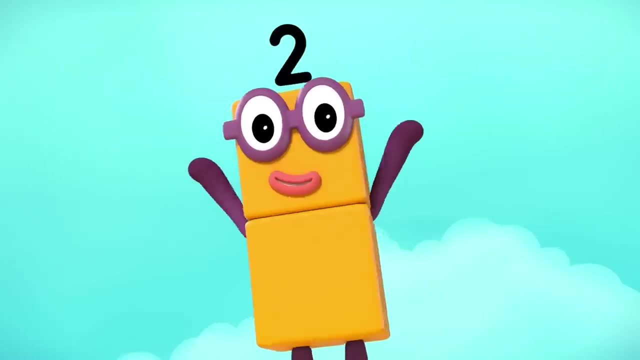 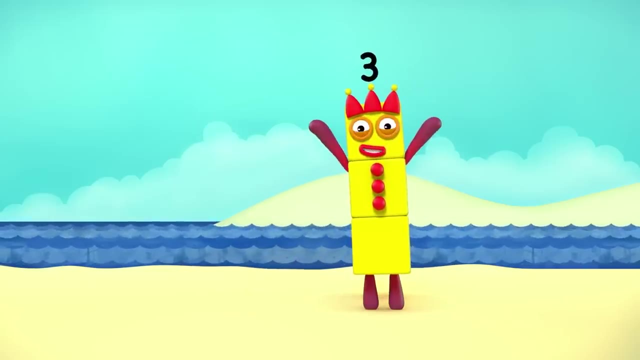 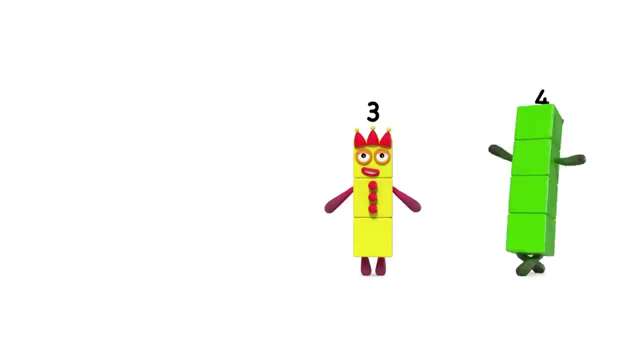 Peek-a-boo, Can you see me, Peek-a-boo? One is smaller than two. I can hide behind you. Two is smaller than three. You can hide behind me, Peek-a-boo. You're hiding behind me Cause I'm smaller than you. no one will find me. 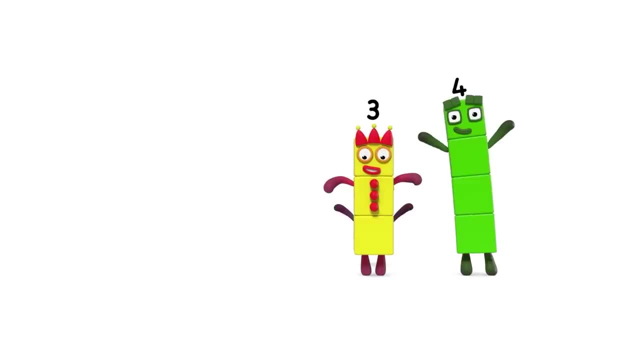 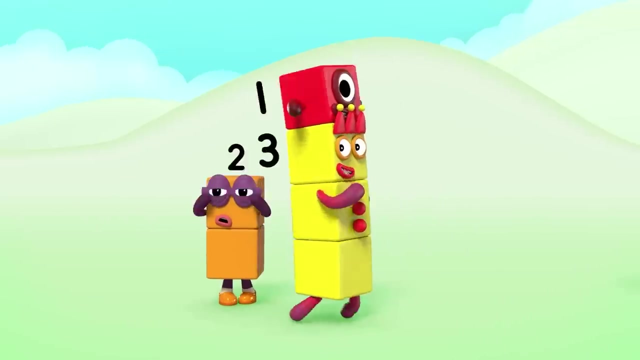 Where have they gone? Go and give us a clue. Can you see me, Peek-a-boo? Can you see me, Peek-a-boo? Two plus one is the same as three. Both of you can hide behind me. Three plus one is the same as four. 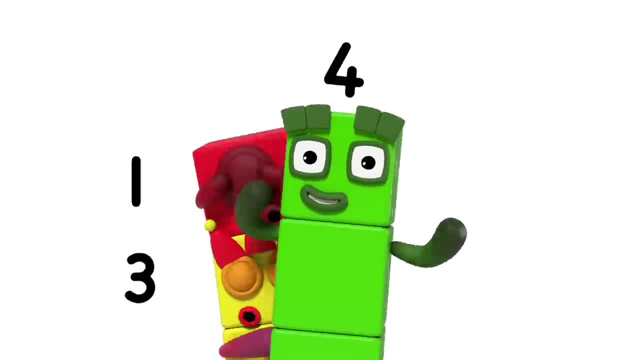 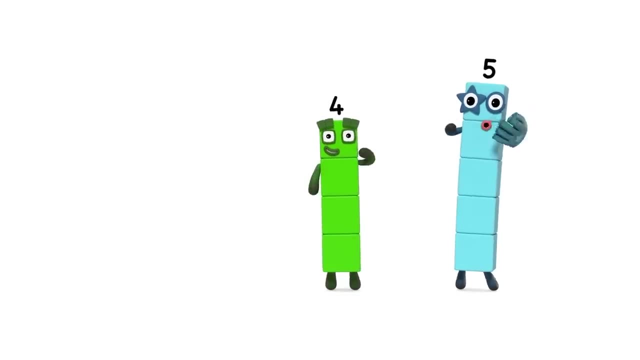 I can hide you both for sure, Peek-a-boo. We're hiding behind you, Cause I'm equal to you. no one will find you. Where have they gone? Go and give us a clue. Can you see me, Peek-a-boo? 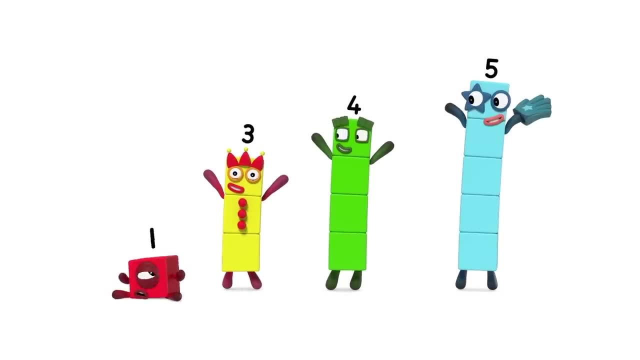 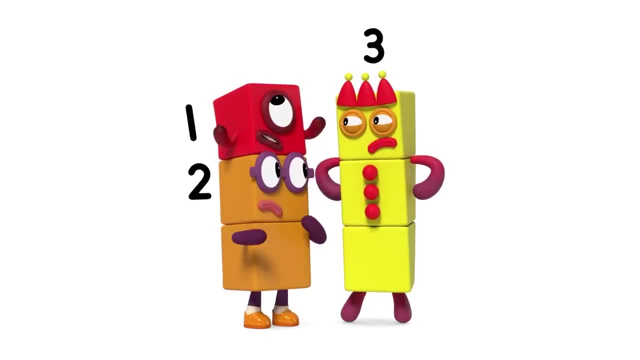 Can you see me Peek-a-boo? Where is the peek-a-boo? It's supposed to be: two plus one is the same as three. Then you can say peek-a-boo, That's too much. Can you see me Peek-a-boo? 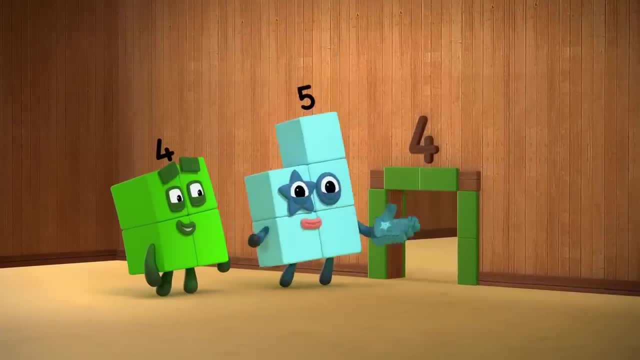 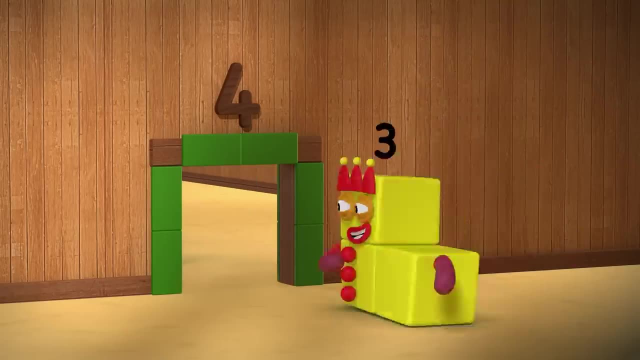 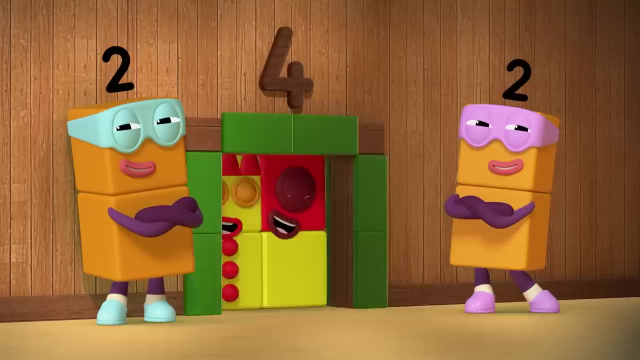 Five is bigger than four. I'll never fit through the door Ow Ow Ow. Three is smaller. Two is smaller than four. I can get through the four door. Three plus one is the same as four. We can fit through the four door. 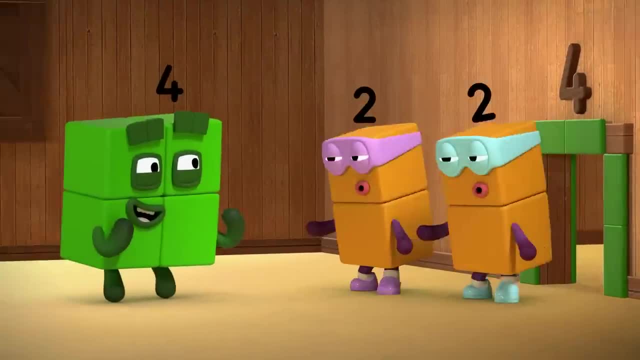 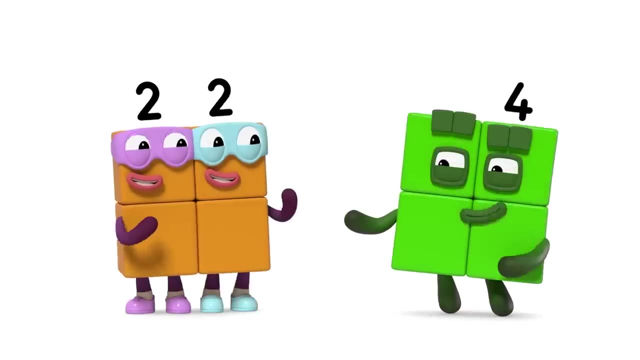 Two plus two is the same as four. Peek-a-boo, We're hiding behind you, Cause I'm equal to you. no one will find you. Where have they gone? Go and give us a clue. Can you see me, Peek-a-boo? 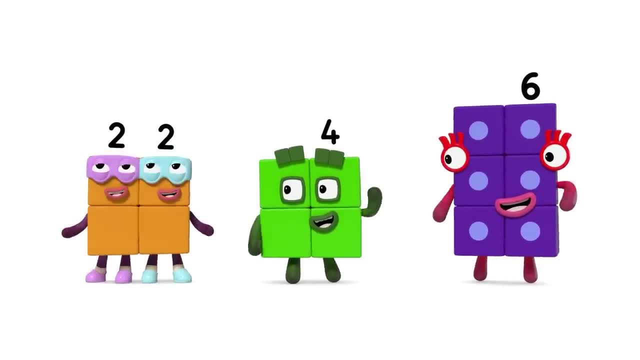 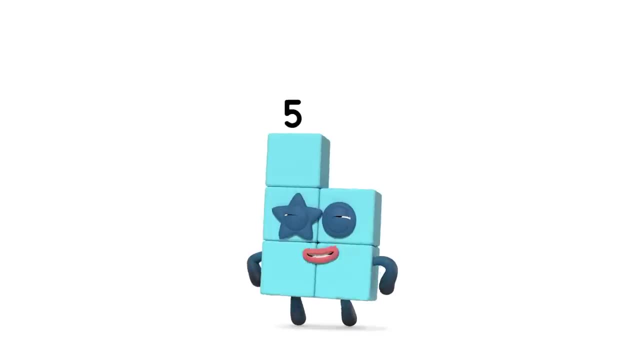 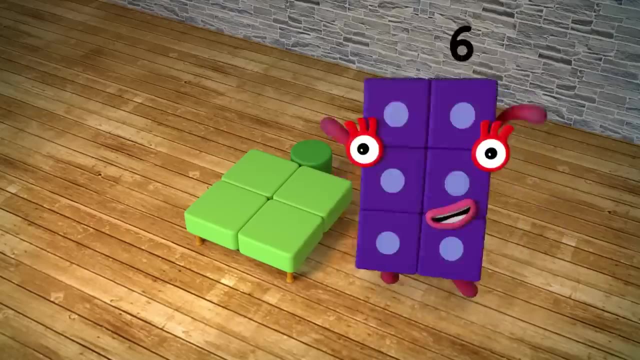 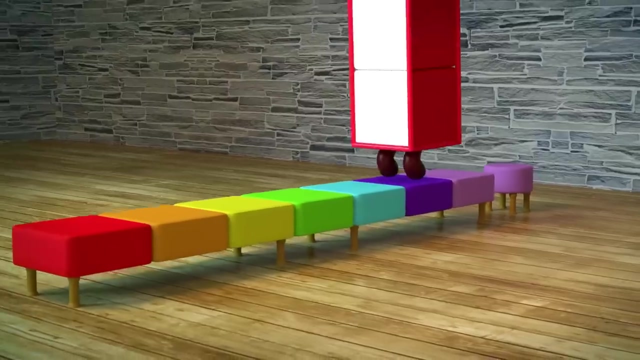 As long as you make the right shape. If you're smaller than me, it'll never work, No matter what shape you make. Six won't fit into four's little bed. I can lie down in ten's bed instead. Seven's bed is too small for ten. 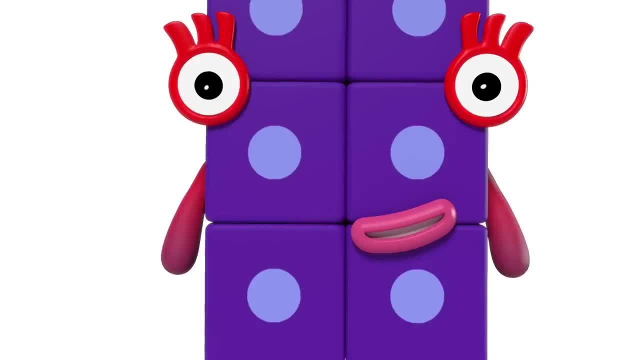 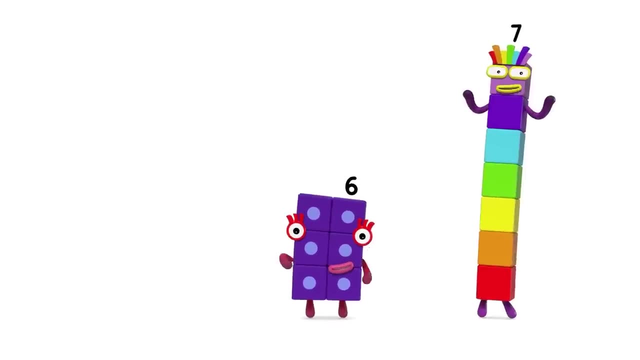 My feet will stick right at the end. Peek-a-boo, I'm hiding behind you. If you're bigger than me, no one will find you. Where have they gone? Go and give us a clue. Can you see me, Peek-a-boo? 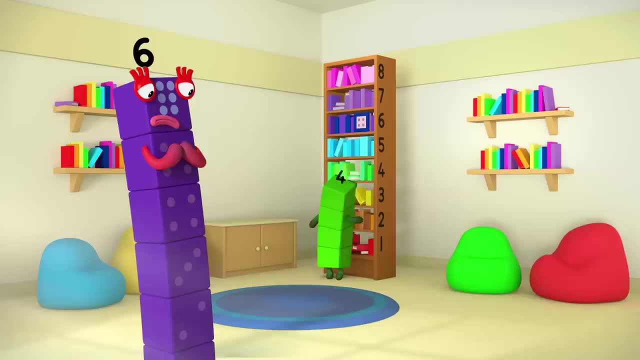 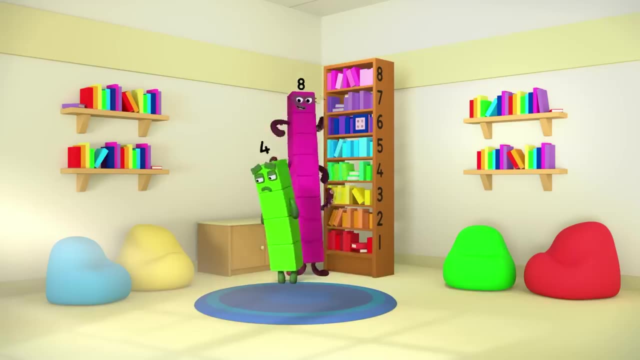 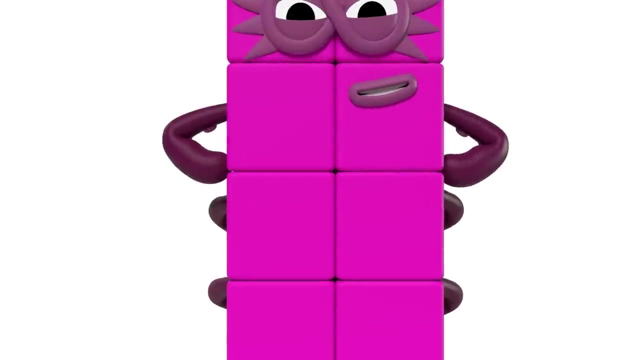 Can you see me, Peek-a-boo? Four can't reach up to six himself. I'll have to leave that book on the shelf. Eight can bend down to reach the book. Six can peek through and take a look, Peek-a-boo, I'm hiding behind you. 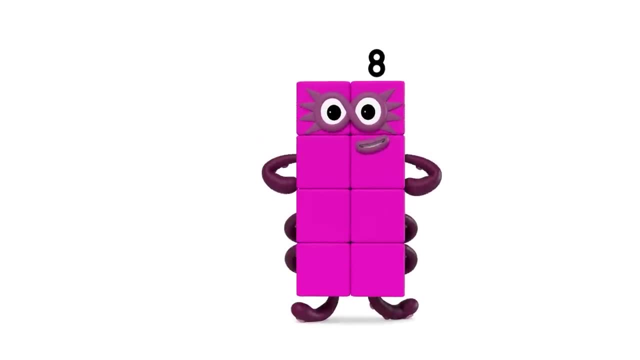 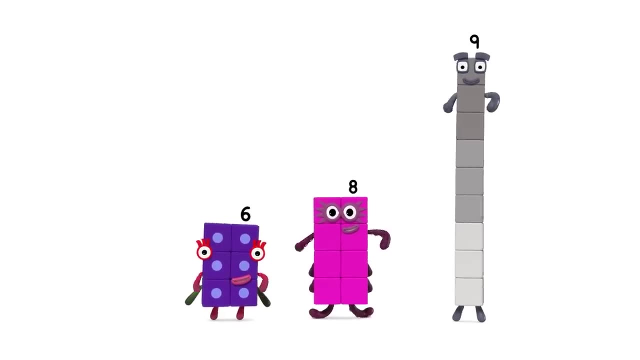 If you're bigger than me, no one can find you. Where have they gone? Go and give us a clue. Can you see me, Peek-a-boo? Can you see me, Peek-a-boo? One is smaller than Fewer than. 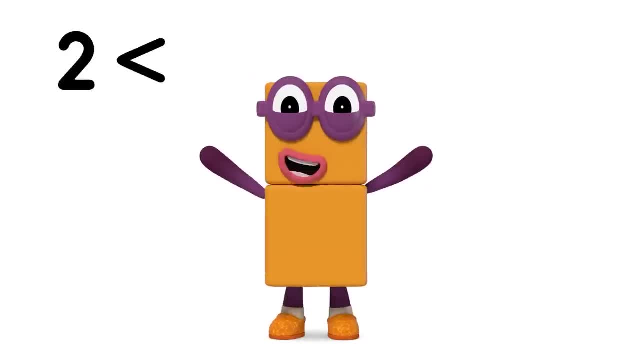 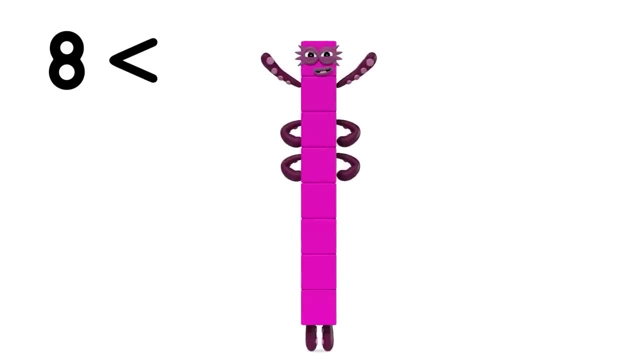 Less than One is less than Two, is less than Three, is less than Four, Five is less than Six, is less than Seven, And eight is less than Nine, is less than Ten And ten is bigger than. 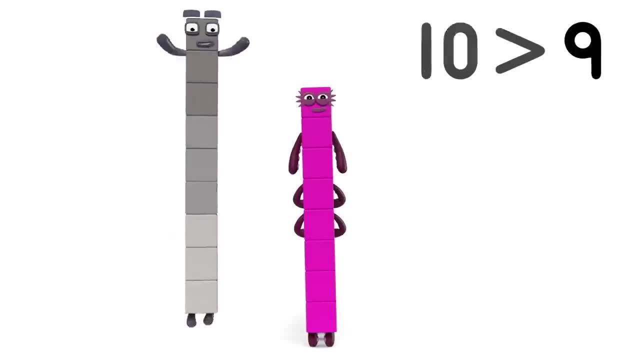 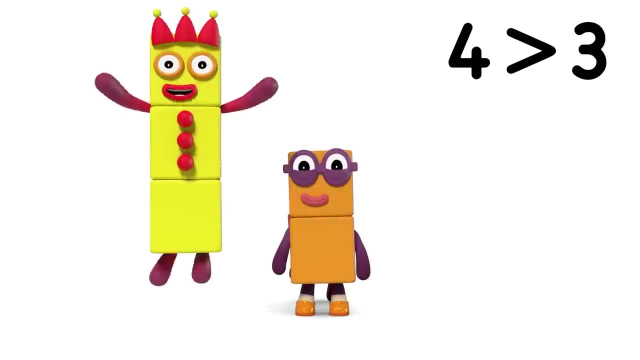 More than Greater than Ten is greater than Nine, is greater than Eight is greater than Seven, Six is greater than Five, is greater than Four, is greater than Three And three is greater than Two is greater than. 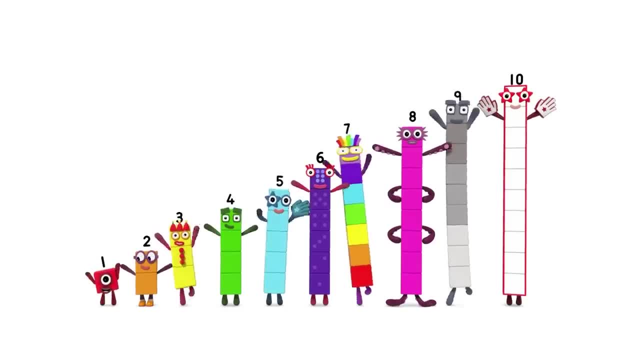 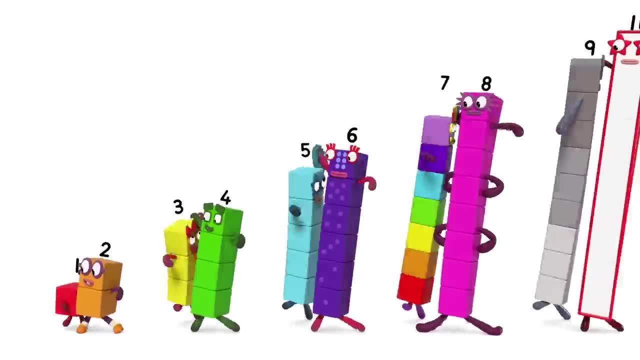 One, Peek-a-boo, I'm hiding behind you Cause I'm bigger than you. no one will find you. Where have they gone? Go and give us a clue. Can you see me, Peek-a-boo? Can you see me, Peek-a-boo?